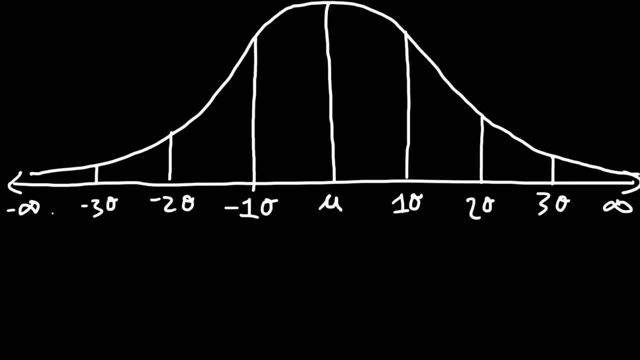 And all the way to the left, negative infinity. Okay Now the area under the curve represents the probability of an event happening between two points. So the probability of an event happening between the mean and the first standard deviation, you can calculate it if you know the 68,, 95,, 99.7 rule. 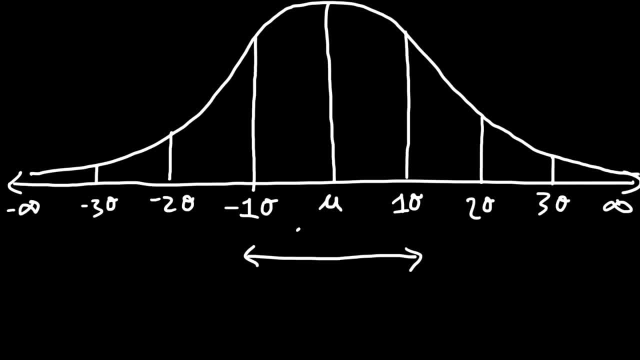 So within the first standard deviation of either side from the mean, there's a 68.2 68% chance that an event will happen in this region. And then, within two standard deviations, the percentage is 95.45%, And then, within three standard deviations of the mean, the percentage is going to be: 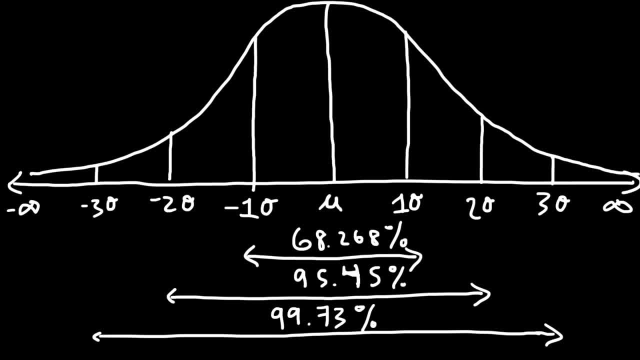 99.73%. Now, I hope that you're taking notes because you're going to need to know these numbers. It's going to help you. It's going to help you solve some problems that are coming up soon. Now, if we take this number- 68.268- and divide it by two, that's going to give us 34.134%. 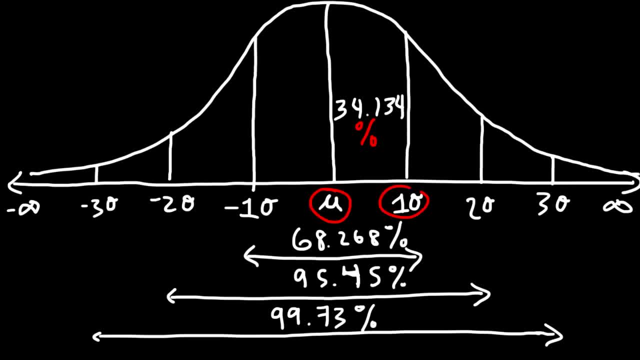 So that's the percentage of finding an event between the mean and the first standard deviation. Now the left side is going to be the same. It's going to be 34.134%. When you're dealing with a normal distribution curve or bell-shaped curve, you can have symmetry. 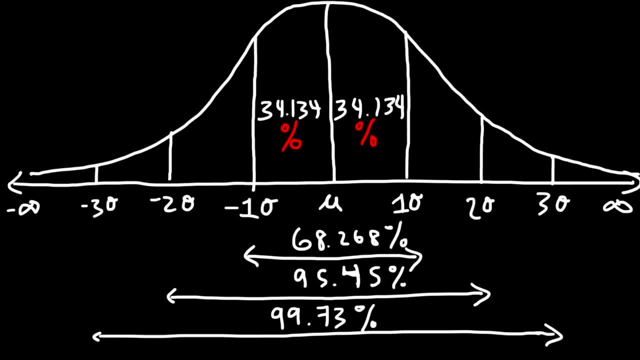 in this problem And keep in mind the area of this region is 0.34134.. It's the percentage as a decimal, So the area is going to be the same as the probability of an event happening within a certain region. Now, 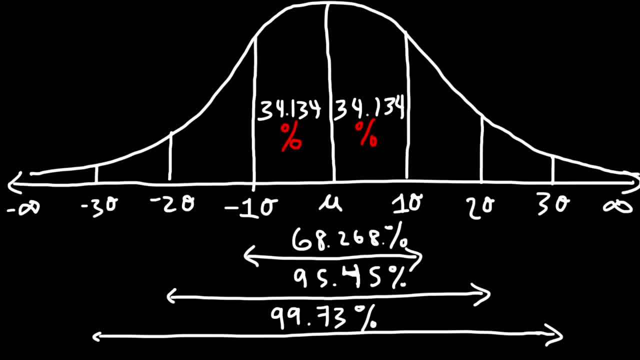 What percentage It goes in this region. If you take the difference between these two numbers- so if you subtract 95.45 by 68.268, that will give you 27.182.. Take that number, divide it by two and you should get 13.591.. 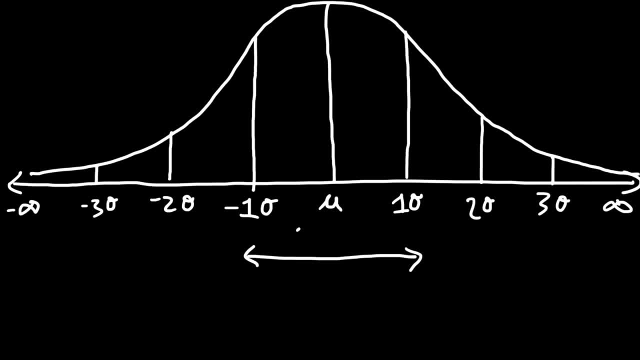 So within the first standard deviation of either side from the mean, there's a 68.2 68% chance that an event will happen in this region. And then, within two standard deviations, the percentage is 95.45%, And then, within three standard deviations of the mean, the percentage is going to be: 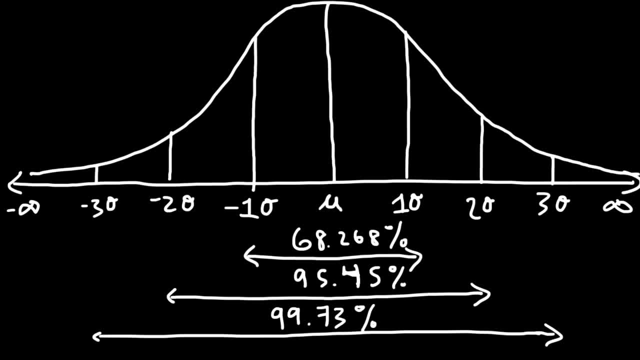 99.73%. Now, I hope that you're taking notes, because you're going to need to know these numbers. It's going to help you- Okay, It's going to help you- solve some problems that are coming up soon. Now, if we take this number- 68.268- and divide it by two, that's going to give us 34.134%. 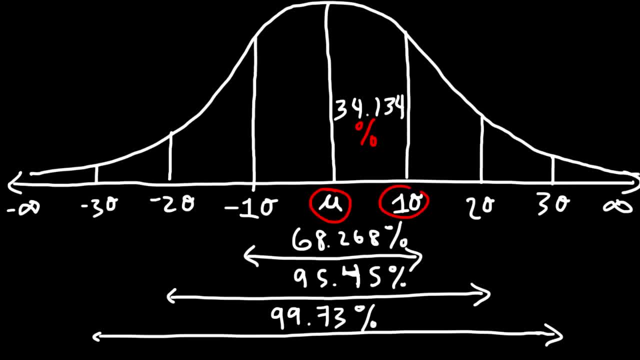 So that's the percentage of finding an event between the mean and the first standard deviation. Now the left side is going to be the same. It's going to be 34.134%. When you're dealing with a normal distribution curve or bell-shaped curve, you can have symmetry in this problem. 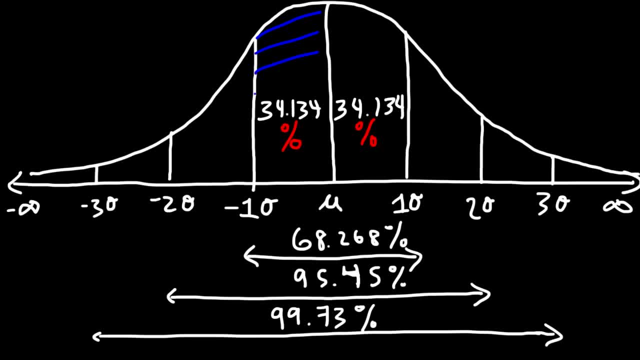 And keep in mind, the area of this region is 0.34134.. It's the percentage as a decimal, So the area is going to be the same as the probability of an event happening within a certain region. Now, what percentage goes in this region? 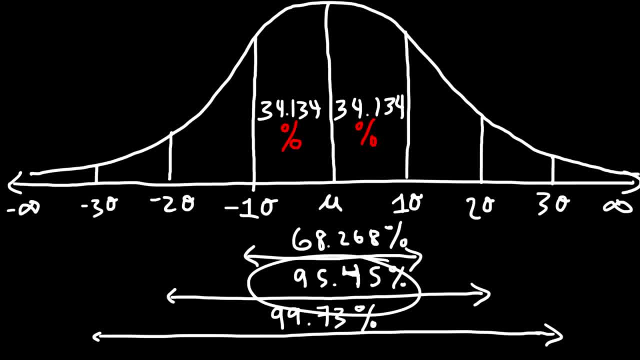 If you take the difference between these two numbers, so if you subtract 95.45 by 68.268,, that will give you 27.182.. Take that number, divide it by two and you should get 13.591.. 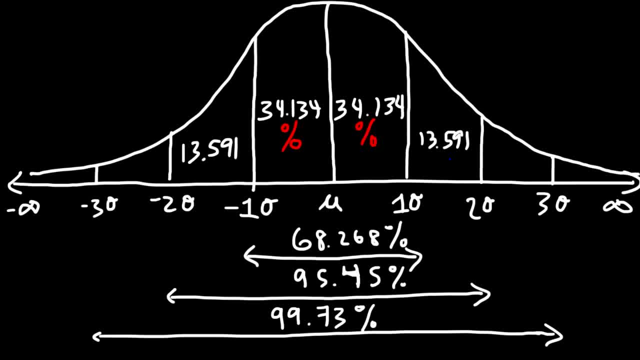 And this number is going to go on both sides. So that's the percentage of an event happening between the first and the second Standard deviations of either side. Now to find the next number, follow the same process. So we're going to subtract these two numbers. 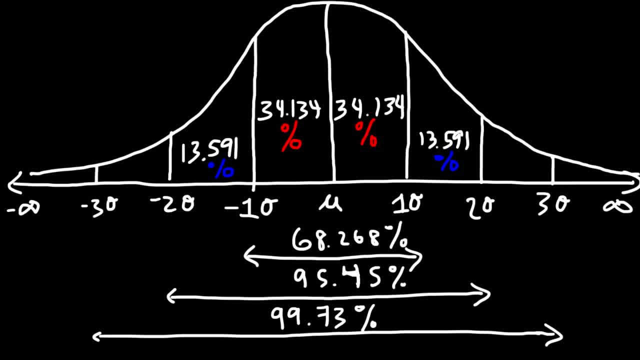 99.73 minus 95.45.. That's 4.28.. Then divide it by two. So the percentage in this region is going to be 2.14%, and the same is true in that region as well. So the percentage in this region is going to be 2.14%, and the same is true in that. 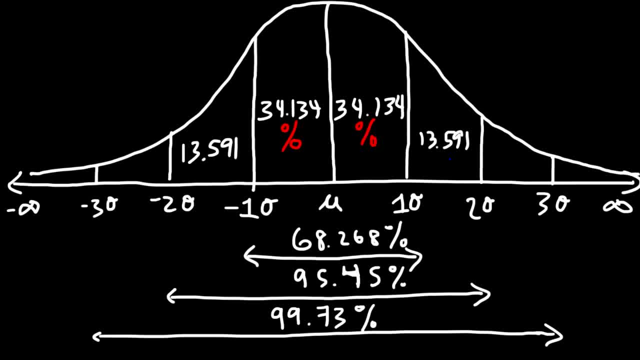 And this number is going to go on both sides. So that's the percentage of an event happening between the first and the second standard deviation. So you can multiply that by two and that's the result. Now to find the next number, follow the same process. 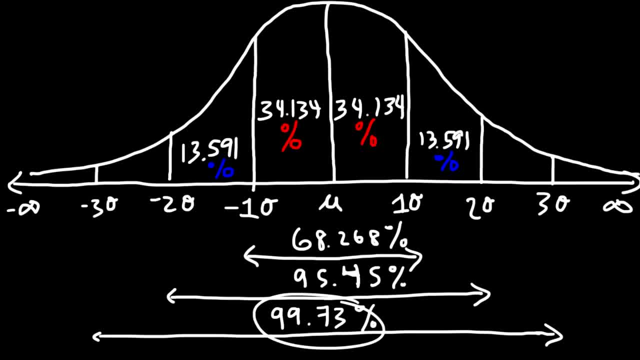 We're going to subtract these numbers, 99.73-95.45 is 4.28.. So that's divided by 2.. So the percentage in this region is 2.14%, And the same is true in that region as well. Then we're going to subtract each number, We're just going to subtract. so this is 5.ーい into the third again. So we've got also a million, and following come Pretty much the ABiyet is 1.000. 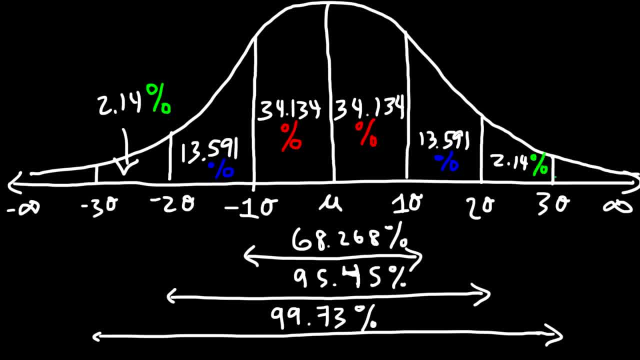 So it goes anytime so far. Then what's the percentage? Now? to find the percentage that goes in those two regions, keep in mind: the total percentage from negative infinity to infinity is 100%. So take 100 and subtract it by 99.73.. 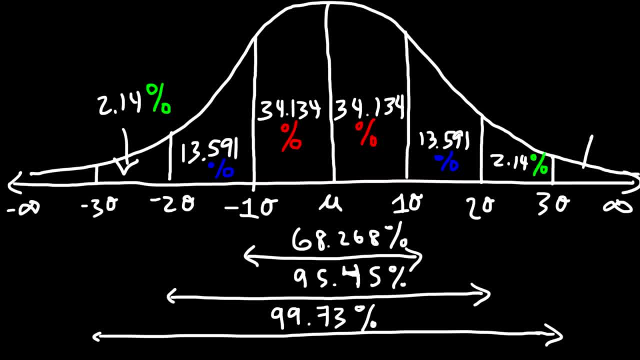 You should get .27.. And when you divide that by 2, the answer in this region is going to be .135%, and the same is true for this area as well. So you may want to take a picture or at least write this down, because you can use this to. 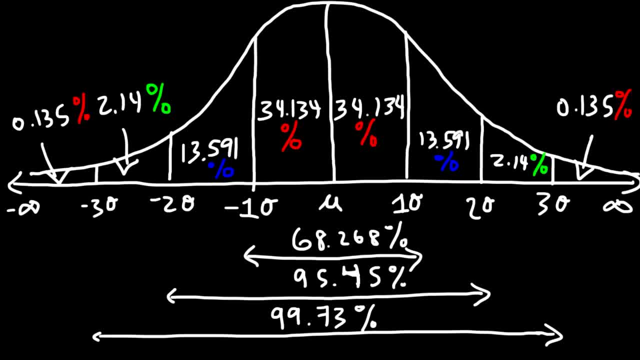 solve problems associated with the normal distribution curve. Now it's important to keep in mind that mu represents the population mean And sigma is the standard deviation. Now, as we said before, The probability of an event happening from negative infinity to infinity is 100%. 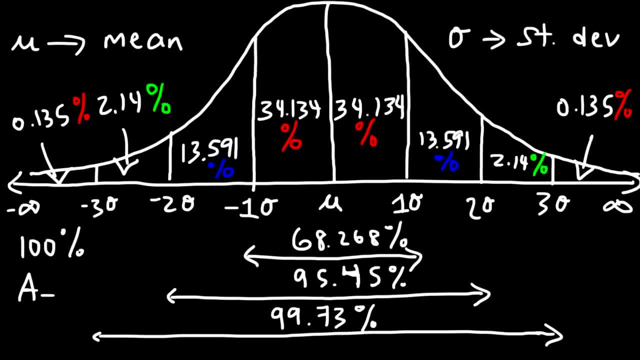 That's the total probability, Which means that the total area of this curve is 1.. So if you add up all of these numbers, you should get 100%, And the left side- everything up to here- has to be 50%. 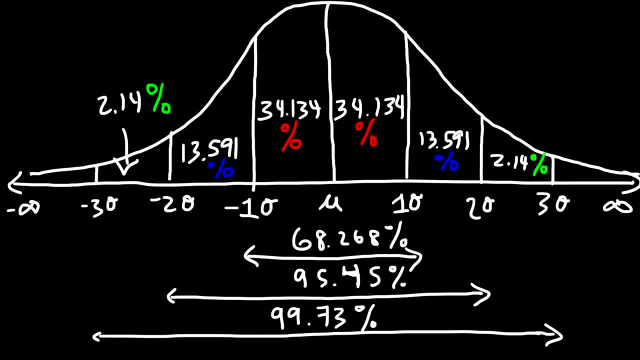 region as well. Now to find the percentage that goes in those two regions, keep in mind: the total percentage from negative infinity to infinity is 100%. So take 100 and subtract it by 99.73.. You should get 0.27. 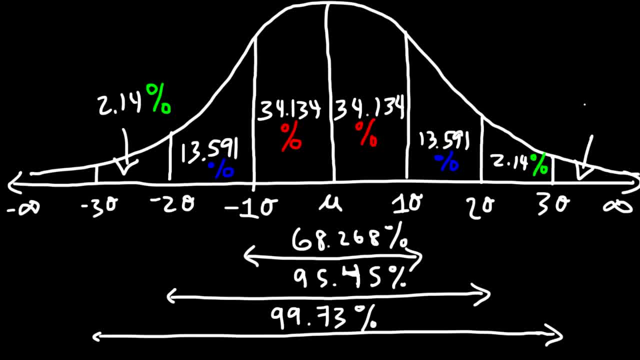 And when you divide that by two, the answer in this region is going to be 0.135%, and the same is true for this area as well. So you may want to take a picture, or at least write this down, because you can use this to. 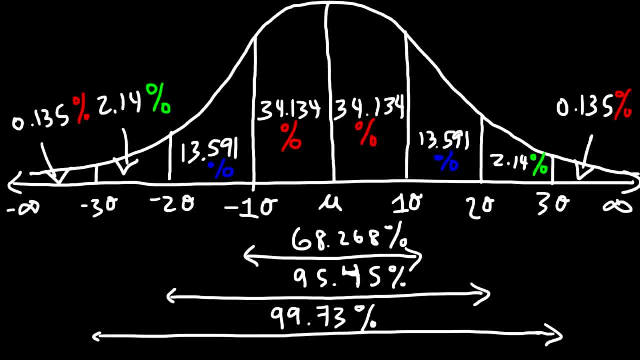 solve problems associated with the normal distribution curve. Now it's important to keep in mind that mu represents the population mean And sigma is the standard deviation. Now, as we said before, the probability of an event happening from negative infinity to infinity Is 100%. 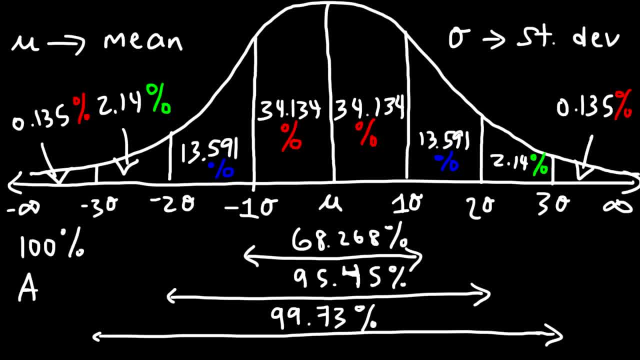 That's the total probability, which means that the total area of this curve is 1.. So if you add up all of these numbers, you should get 100%, And the left side- everything up to here- has to be 50%, which is 0.5 as a decimal. 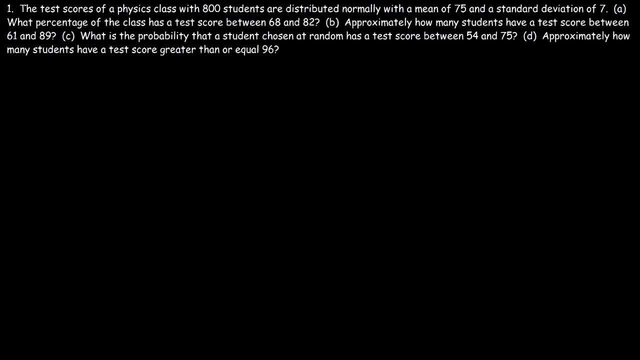 So now let's work on some practice problems. Number one: the test scores of a physics class with 800 students are distributed normally with a mean of 75 and a standard deviation of 7.. Part A: what percentage of the class has a test score between 68 and 82?? 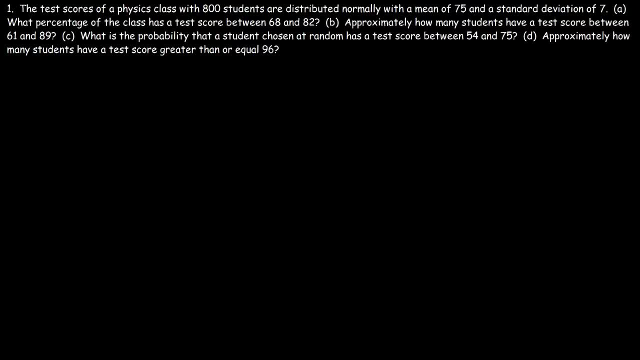 So feel free to pause the video and work on this problem Now. what I'm going to do first is I'm going to draw a picture. Okay, That's similar to the picture that I had before, But instead of using symbols such as mu and sigma, I'm going to use numbers. 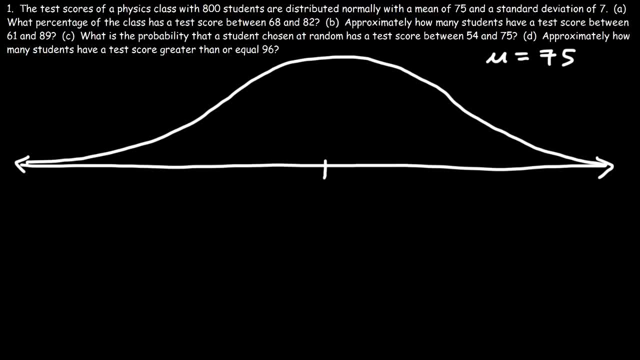 Now we said that the mean is 75 and the standard deviation is 7.. So the first thing I would recommend doing is putting the mean right in the middle, Then one standard deviation away from the mean. We're going to put the numbers as well. 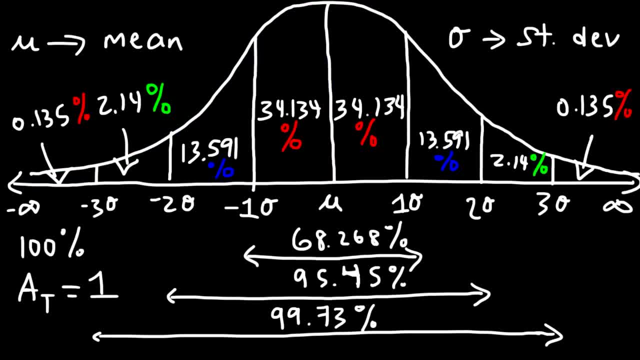 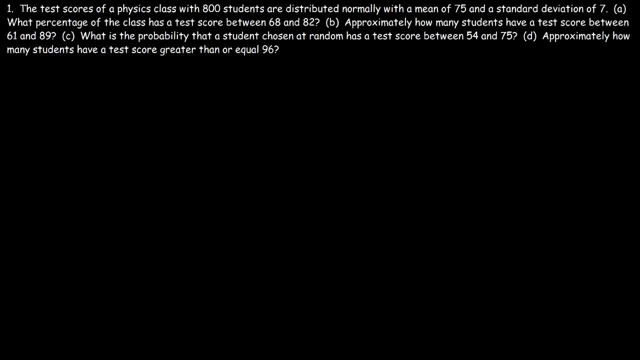 Which is .5 as a decimal. So now let's work on some practice problems. Number 1. The test scores of a physics class with 800 students are distributed normally with a mean of 75 and a standard deviation of 7.. Part A: What percentage of the class has a test score between 68 and 82?? 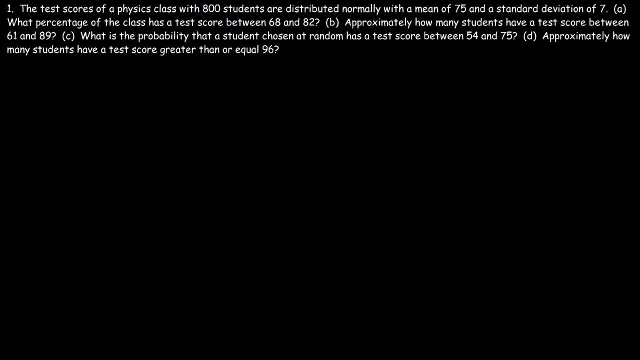 So feel free to pause the video and work on this problem Now. what I'm going to do first Is I'm going to draw a picture That's similar to the picture that I had before, But instead of using symbols such as mu and sigma. 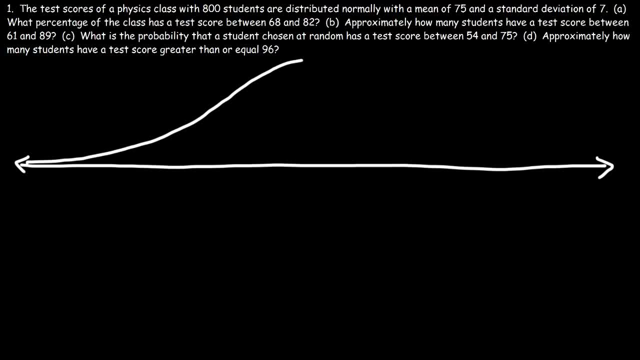 I'm going to use numbers Now. we said that the mean is 75. And the standard deviation is 7.. So the first thing I would recommend doing Is putting the mean right in the middle. So I'm going to draw a picture. 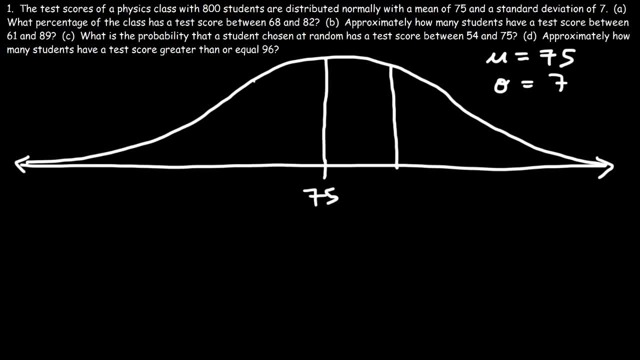 Then one standard deviation away from the mean. We're going to put the numbers as well. So we're going to add 7 to 75.. 75 plus 7 is 82. And 75 minus 7 is 68.. Now let's move another standard deviation away from the next number. 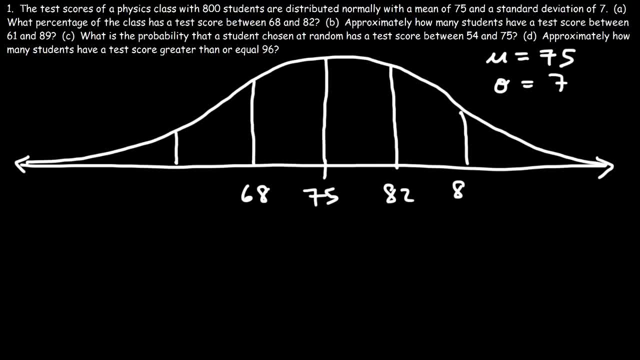 From 82 and 68.. So 82 plus 7 is 89.. 68.. Minus 7 is 61.. Now let's do it one more time: 89 plus 7 is 96.. 61 minus 7 is 54.. 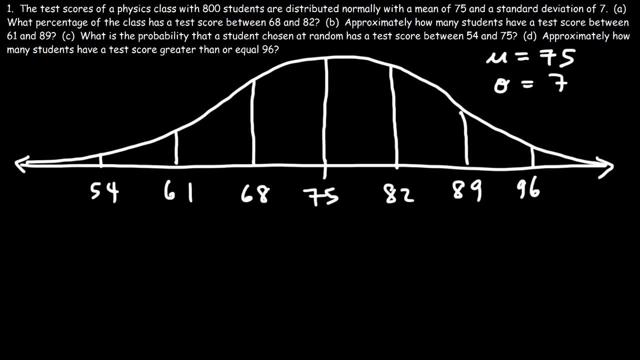 And we could stop here. Now let's put the appropriate percentages in each region. So we know that within the first standard deviation It's going to be 34.134%, And then, between the first and the second standard deviation, It's going to be 13.591%. 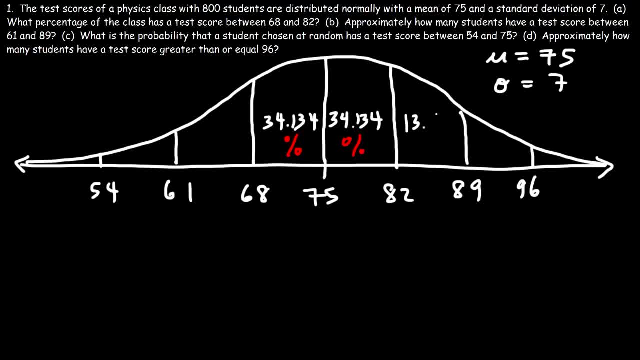 And between the second and the third, It's going to be 2.14%, And between the second and the third, It's going to be 2.14%- 31.6%, And then between the second and the third, It's going to be 2.14%. 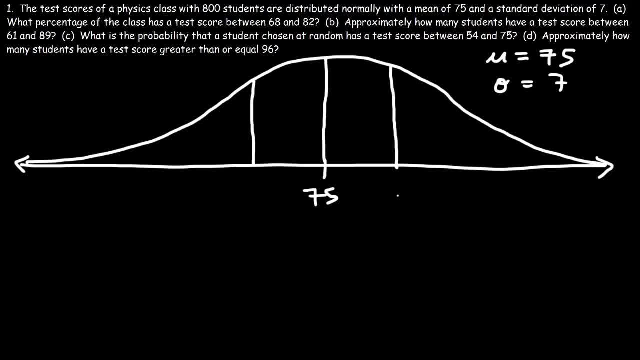 So we're going to add 7 to 75.. 75 plus 7 is 82.. And 75 minus 7 is 68.. Now let's move another standard deviation away from the next number, from 82 and 68.. 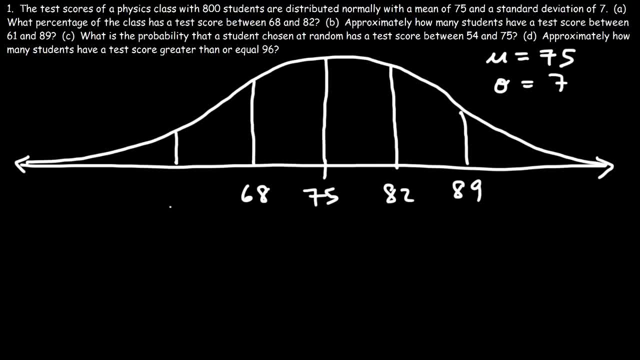 So 82 plus 7 is 89.. 68 minus 7 is 61.. Now let's do it one more time: 89 plus 7 is 96.. 61 minus 7 is 54. And we could stop here. 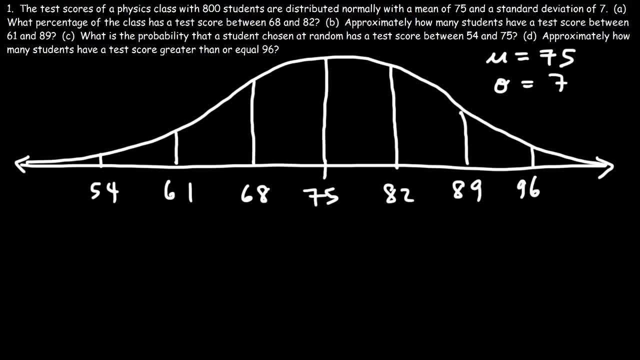 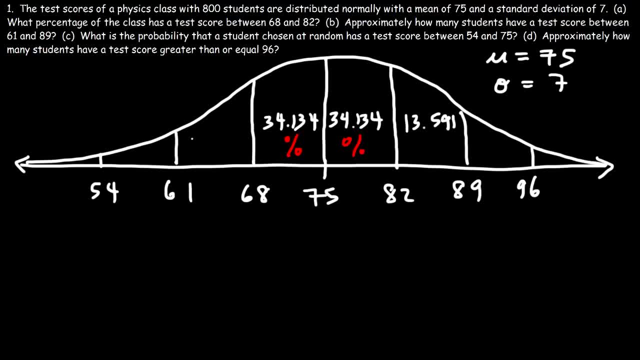 Good, Great, Great 行いて. Thank you, Thanks, Thank you, Take care, Bye. And between the second and the third it's going to be 2.14% And then, for this region, 0.135%. 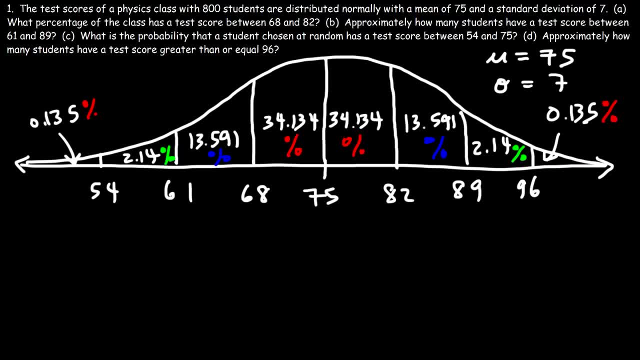 So now we have everything that we need in order to get the answer. So let's calculate the probability, or the percentage of the class that has a test score between 68 and 82.. So x is going to be a random continuous variable that can vary beyond 75 or less than 75. 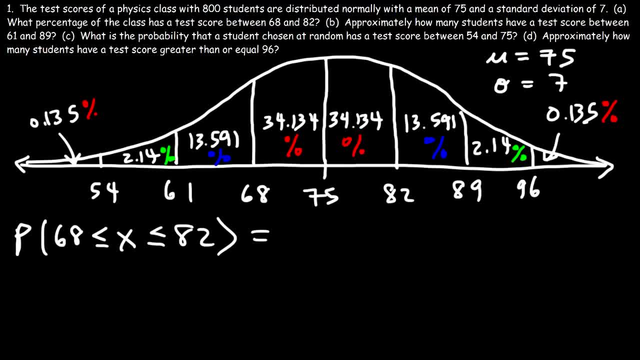 Now all we need to do to get the answer is basically find the answer. So we're going to find the area under the curve between these two numbers. So we've got to find the area of the shaded region. So all we need to do is simply add up the percentages between 68 and 82.. 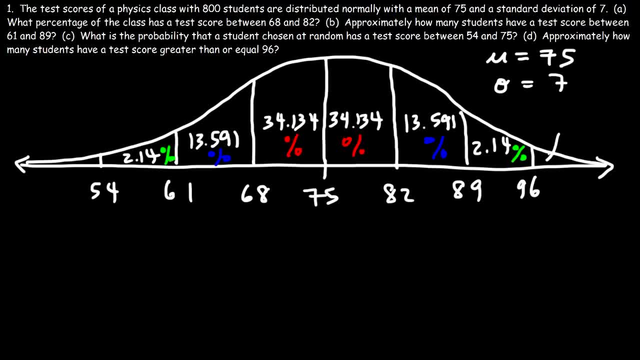 And then for this region, 0.135%. So now we have everything that we need in order to get the answer. So let's calculate the probability, or the percentage of the class that has a test score between 68 and 82.. So X is going to be a random continuous variable that can vary beyond 75 or less than 75. 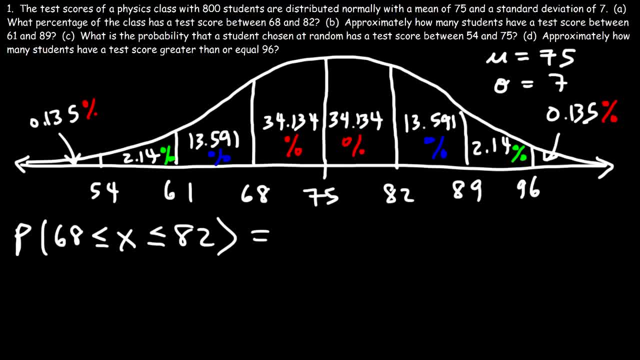 Now all we need to do to get the answer is basically find the area under the curve between these two numbers. So we've got to find the area of the shaded region. Okay, So all we need to do is simply add up the percentages between 68 and 82.. 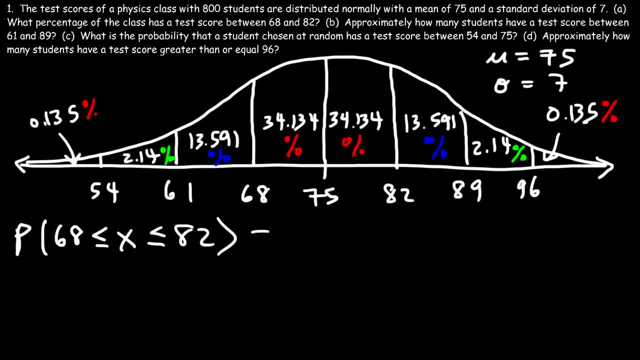 So it's going to be 34.134 plus another 34.134.. So that's going to be 68.268%. So that's the percentage of the class that has a test score between 68 and 82.. Okay, Now there's a formula that you could use to get the same answer, in fact, a more accurate. 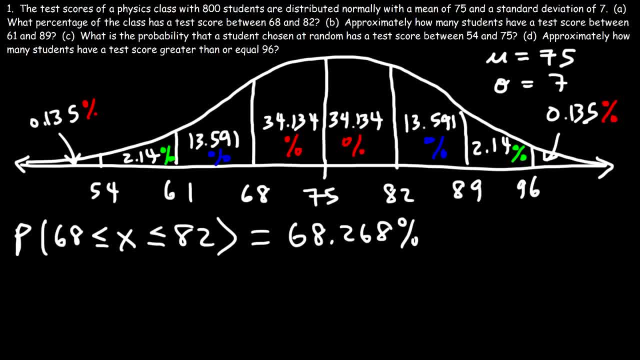 answer using calculus. Now, if you're watching this video and if you haven't taken a calculus class, don't worry about it, because the formula that I'm going to show you, you can easily use it with the appropriate calculator. And if you don't have a calculator, I can show you how to use it with an online calculator. 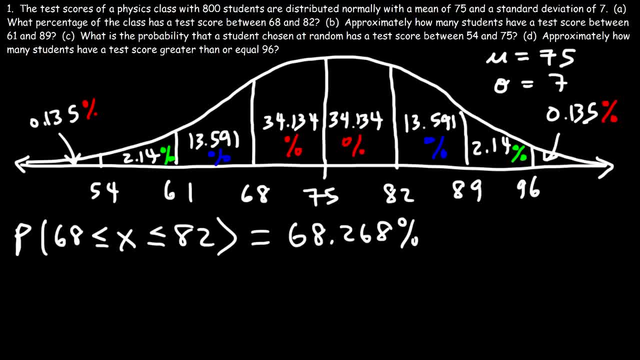 at Wolfram Alpha. So here's the formula that you need: The probability of finding an event between A and B. Okay, Okay, So the probability of finding an event between A and B is going to be the definite integral from A to B, E. E is the inverse of the natural log function and then raised to the negative. 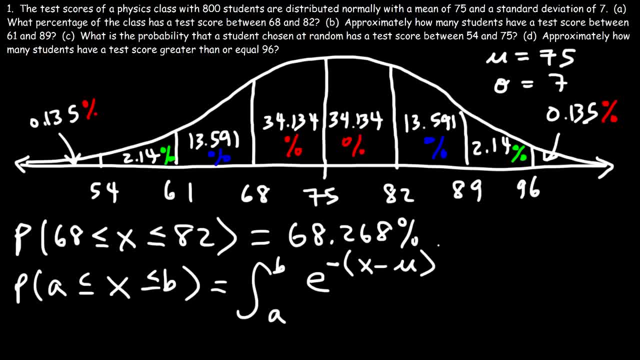 X minus the population mean squared divided by 2 times the square of sigma or the standard deviation, And this is all divided by sigma times the square root of 2 pi, And then we have a DX symbol here. Okay, Now all you need to do is plug in the population mean which you have, that's 75.. 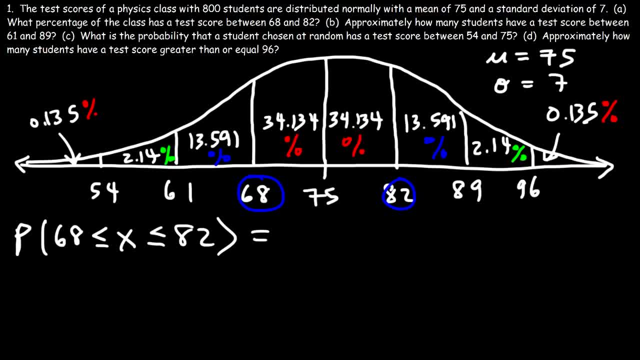 So it's going to be 34.134 plus another 34.134.. So that's going to be 68.268%. So that's the percentage of the class that has a test score between 68 and 82.. Now there's a formula that you could use to get the same answer- in fact a more accurate answer, using calculus. 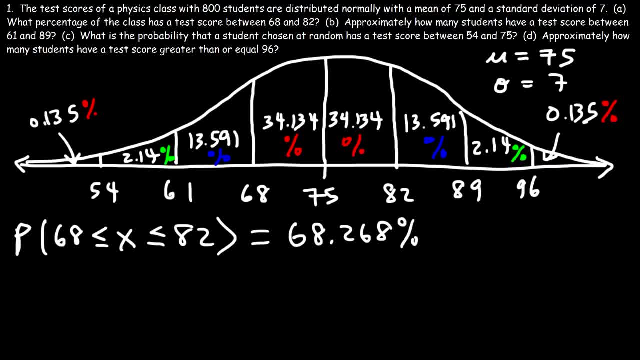 Now, if you're watching this video and if you haven't taken a calculus class, don't worry about it, Because the formula that I'm going to show you, you can easily use it with the appropriate calculator. And if you don't have a calculator, I can show you how to use it with an online calculator. 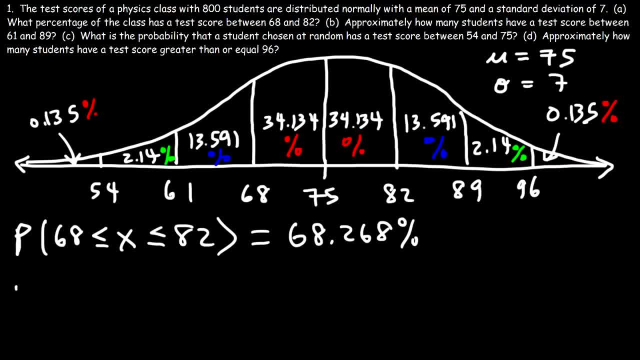 At WolframAlpha. So here's the formula that you need. The probability of finding an event between A and B is going to be the definite integral from A to B, E. E is the inverse of the natural log function And then raised to the negative x minus the population mean squared divided by 2 times the square of sigma. 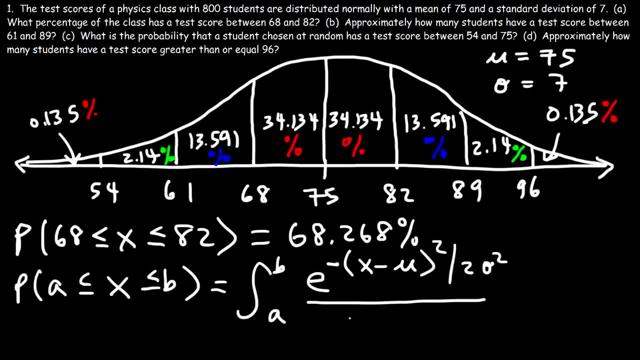 Or the standard deviation, And this is all divided by Sigma times the square root of 2 pi, And then we have a dx symbol here. Now all you need to do is plug in the population mean which you have, that's 75.. 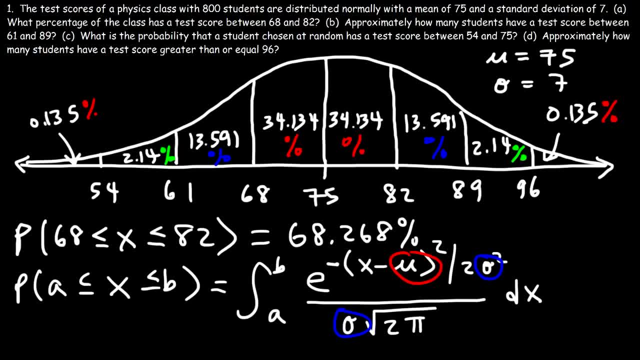 You also need to plug in the standard deviation, which is 7. And then plug in A and B. In this case, A is 68,, B is 82. And then just type that into the calculator and that should give you the answer. 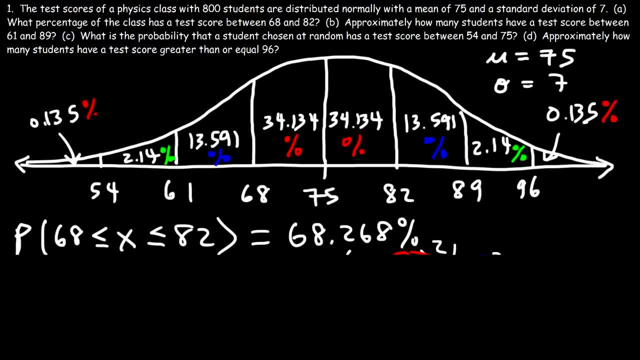 So let's go ahead and do that. So the percentage of students with a test score between 68 and 82 is going to be the definite integral from 68 to 82.. And then it's going to be E raised to the negative: x minus 75 squared divided by 2.. 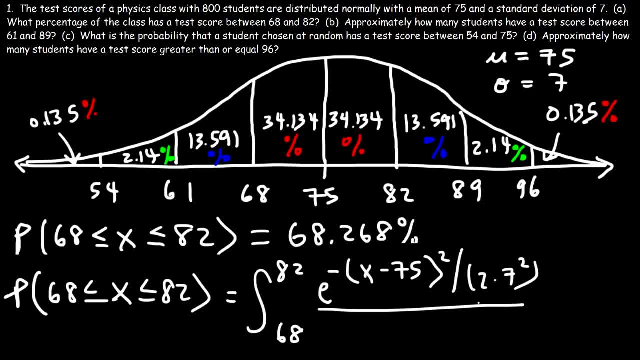 2 times 7 squared, divided by 7 times the square root of 2 pi dx. So make sure to use these parentheses that I'm showing you when you're plugging into your graphing calculator. I'm going to show you how to use Wolfram Alpha towards the end of this video. 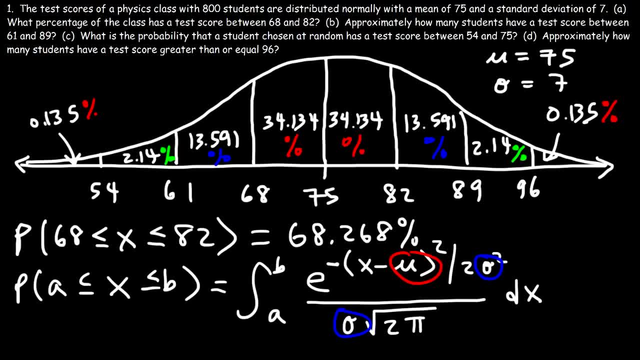 You also need to plug in the standard deviation, which is 7. And then plug in A and B. In this case, A is 68,, B is 82. And then just type that into the calculator and that should give you the answer. 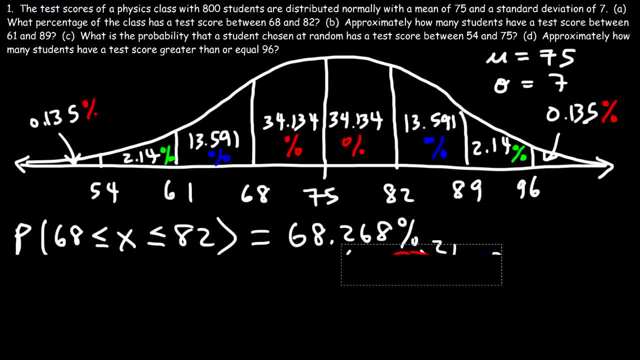 So let's go ahead and do that, Okay, Okay, Okay. So the percentage of students with a test score between 68 and 82 is going to be the definite integral from 68 to 82.. And then it's going to be E raised to the negative, X minus 75, squared divided by 2. 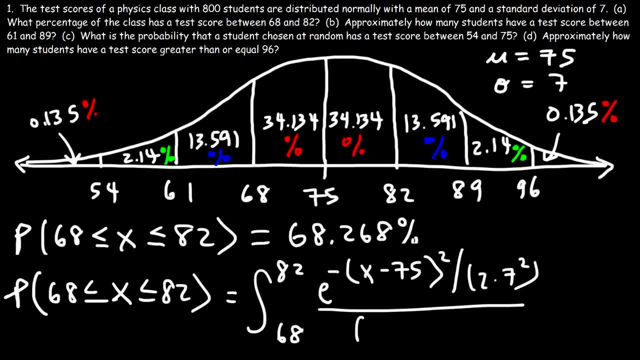 times 7 squared, divided by 7. 7 times the square root of 2 pi dx. So make sure to use these parentheses that I'm showing you when you're plugging into your graphing calculator. I'm going to show you how to use Wolfram Alpha towards the end of this video. 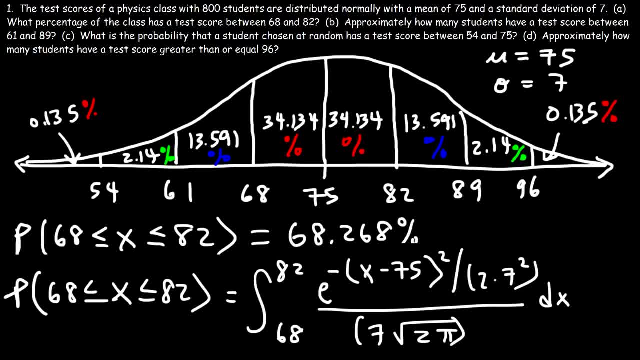 So you can look for it then. So let's go ahead and plug this in. It's going to take me a while to type this in, so bear with me for one moment. It's going to take a while for the calculator to get the answer to. 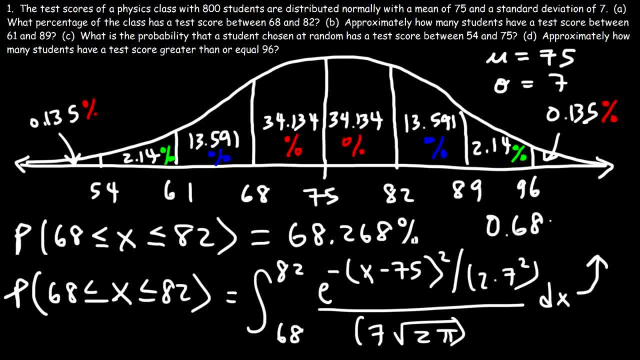 So what I got is 0.67.. So if you multiply that by 100, that's going to be 68.268949%. So, as you can see, these two answers are not exactly the same, but they're close enough. 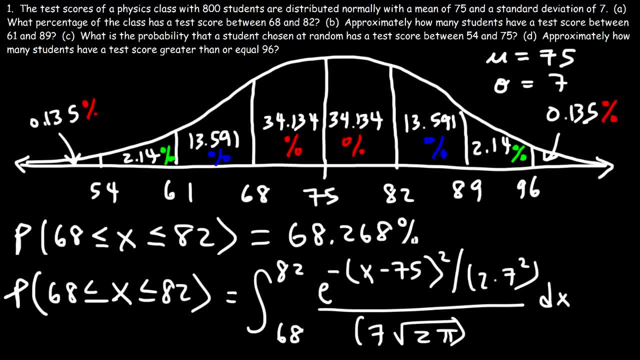 So you can look for it then. So let's go ahead and plug this in. It's going to take me a while to type this in, so bear with me for one moment, And it's going to take a while for the calculator to get the answer to. 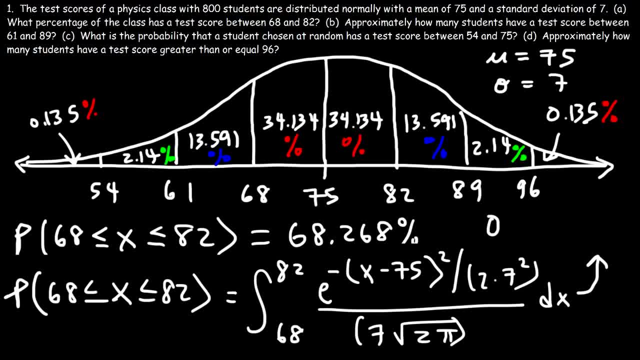 So what I got is 0.68.. 2, 6, 8,, 9,, 4, 9.. So if you multiply that by 100, that's going to be 68.268949%. So, as you can see, these two answers are not exactly the same, but they're close enough. 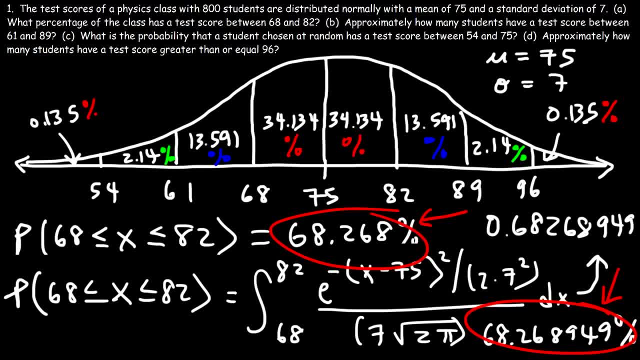 So this is an approximation And this answer is more accurate to the exact answer. So technically it should be like 68.269 instead of 268. But if you round it to 68.3, then you should be fine. Now let's move on to our next problem, or the next part of this problem. 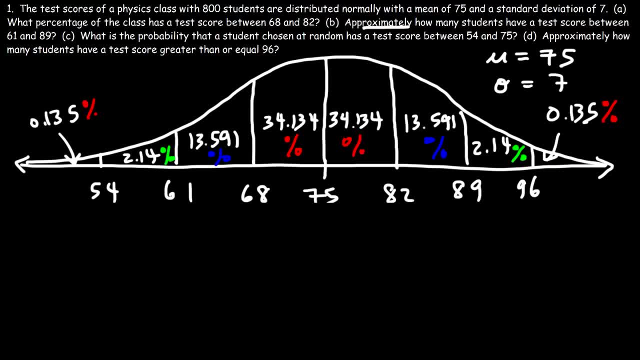 That is part B. Approximately, how many students have a test score between 61 and 89?? So we're not looking for it. We're looking for a percentage, but rather the number of students, And keep in mind we have a total of 800 students in this class. 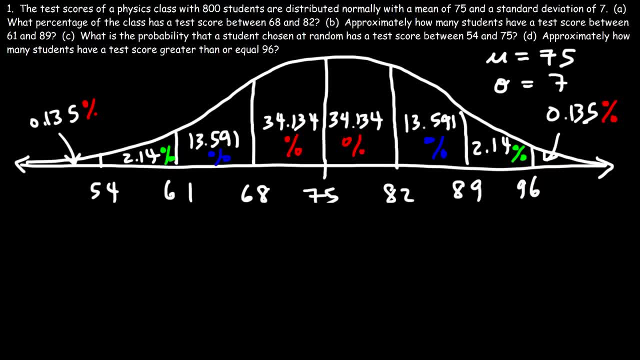 So first let's find the percentage, as we did in part A. So the percentage of students with a test score between 61 and 89 is going to be. So we're starting at 61, and we wish to end at 89.. 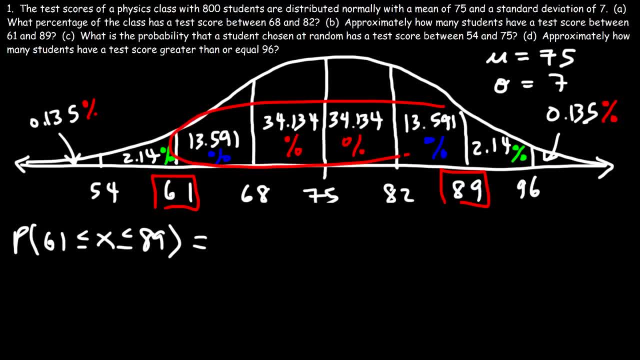 So we need to find the area under the curve For that entire region. So basically we need to add those four numbers. So we're going to add 13.591 plus 34.134, plus 34.134 again, and then another 13.591. 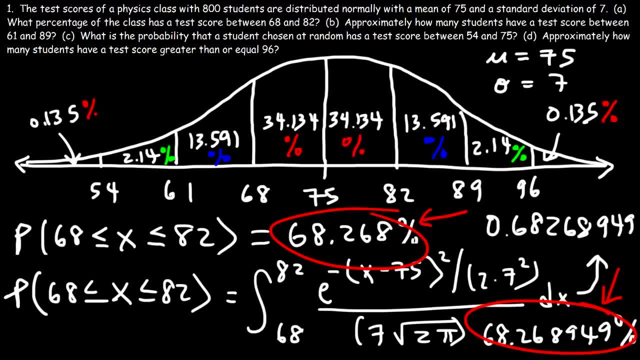 So this is an approximation And this answer is more accurate. So technically it should be like 68.269 instead of 268, but if you round it to 68.3, then you should be fine. Now let's move on to our next problem, or the next part of this problem. 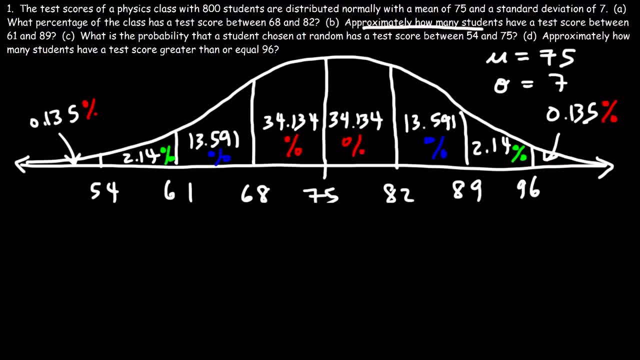 That is part B. Approximately, how many students have a test score between 61 and 89?? So we're not looking for a percentage, but rather the number of students, And keep in mind we have a total of 800 students in this class. 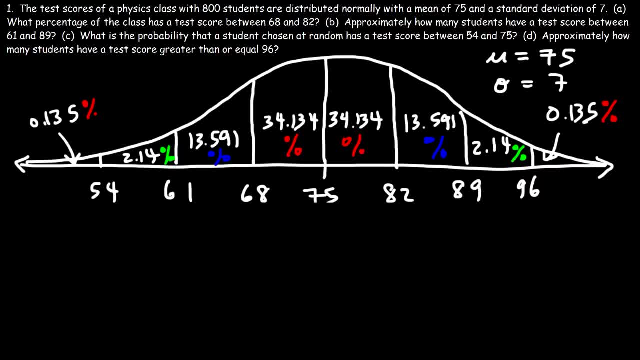 So first let's find the percentage, as we did in part A. So the percentage of students with a test score between 61 and 89 is going to be. So we're starting at 61, and we wish to end at 89.. 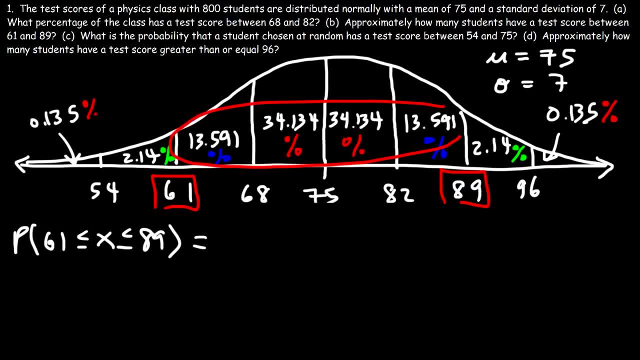 So we need to find the area. Okay, So we'll just need to add that part B and get that number together. So, as you can see here, this is the average. I'm going to do that right here. So, instead of finding the number for the entire region, you're gonna need to find the 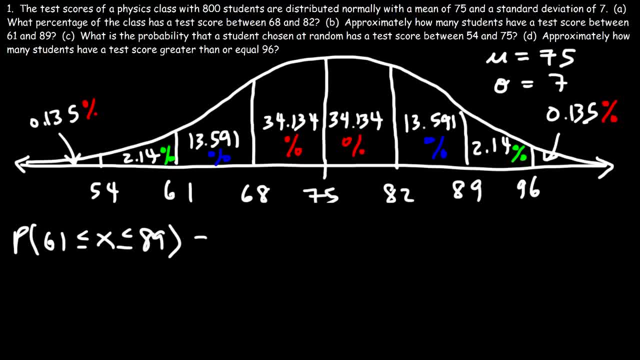 number for the entire region. So basically we need to add those four numbers. So we're going to add 13.591 plus 34.134, plus 34.134 again, And then another 13.591.. And you should get approximately 95.45%. 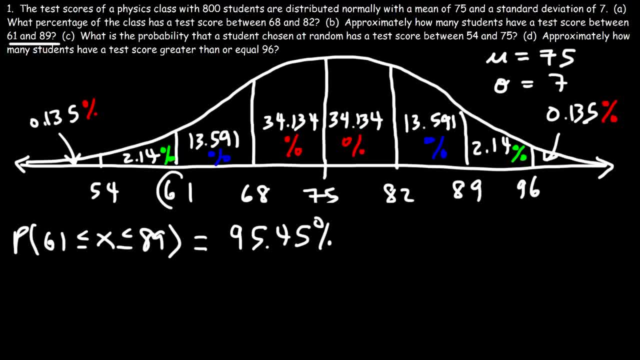 Okay, because these two numbers they're within two standard deviations of the mean, So that's always going to be about 95.45% whenever you have that situation. Now let's confirm this answer with a calculator. So we're going to evaluate the definite integral from 61 to 89,. 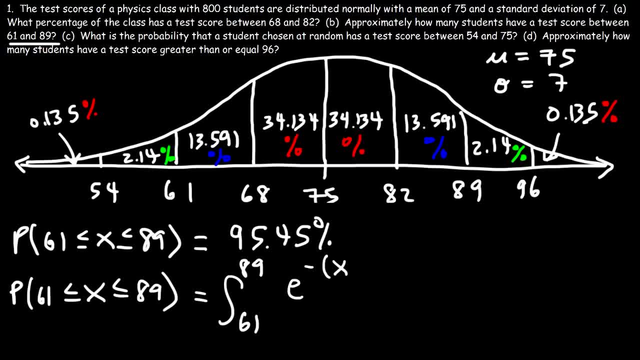 and then it's going to be e raised to the negative, x minus 75 squared divided by 2 times 7 squared divided by 7 times the square root of 2 pi. So notice that this portion doesn't change because the mean and the standard deviation is the same for part a and b. 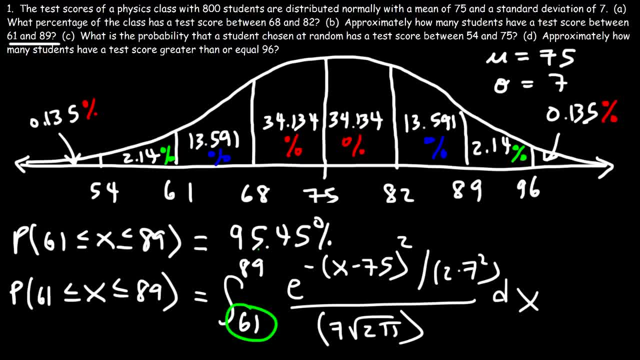 The only thing that's changing is the limits of integration a and b. That's all we need to change in this problem, So go ahead and plug that in. If you don't know how, I'll show you later at the end of this video. 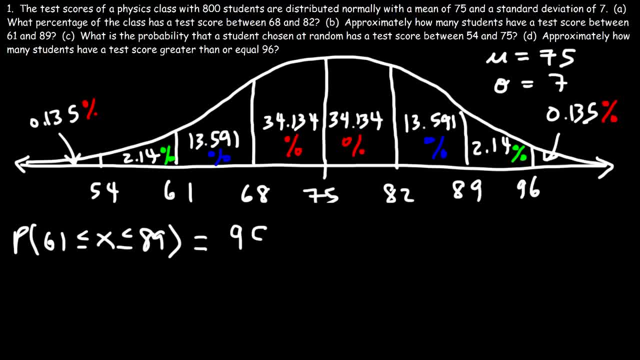 And you should get approximately 95.45%, Because these two numbers They're within two standard deviations of the mean, So that's always going to be about 95.45% Whenever you have that situation. Now let's confirm this answer with a calculator. 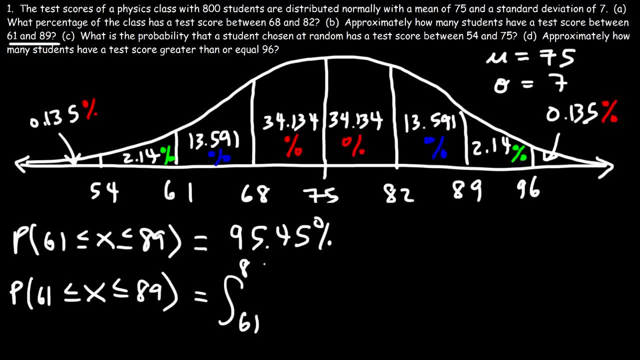 So we're going to evaluate the definite integral from 61 to 89.. And then it's going to be e raised to the negative x minus 75. So we're going to have Square divided by 2 times 7, squared Divided by 7 times the square root of 2 pi. 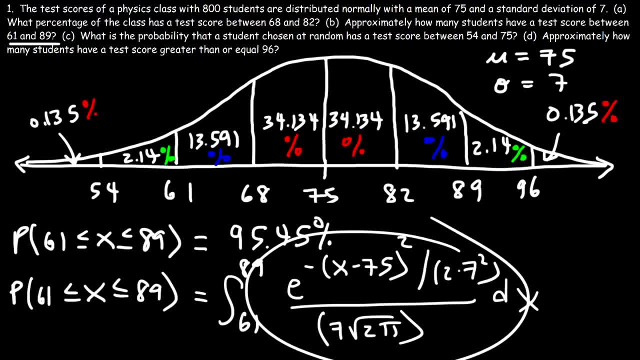 So notice that this portion doesn't change, Because the mean and the standard deviation is the same for part A and B. The only thing that's changing is the limits of integration A and B. That's all we need to change in this problem. 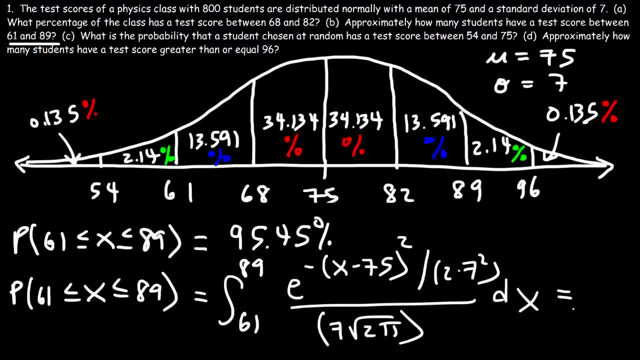 So go ahead and plug that in. If you don't know how, I'll show you later at the end of this video. This calculator takes about 5 seconds to get the answer, So I got 0.9545.. So that's approximately 95.44997%. 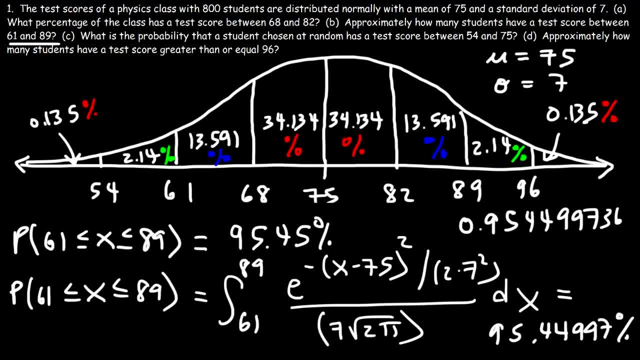 If you multiply this by 100. So this answer is more accurate, But nevertheless, this is a good estimate of this answer. It rounds pretty well. Now, this is not the final answer for part B, So what this means is that 95.45% of the class. 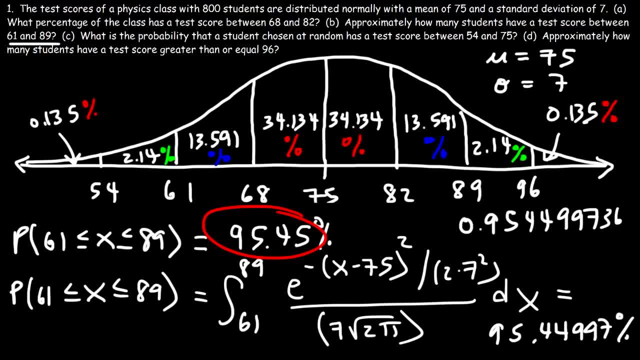 Has a negative x, So that's approximately 95.44997%. It has a test score between 61 and 89. Now there's 800 students. So what's 95.45% of 800?? So what I'm going to do is take this number. 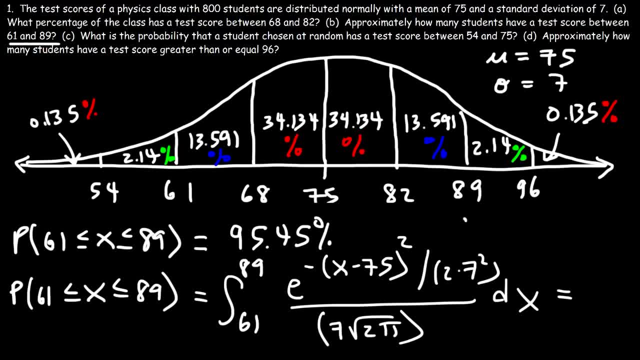 This calculator takes about 5 seconds to get the answer. So I got 0.954499736.. So that's approximately 95.44997% if you multiply this by 100.. So this answer is more accurate, but nevertheless, this is a good estimate of this answer. 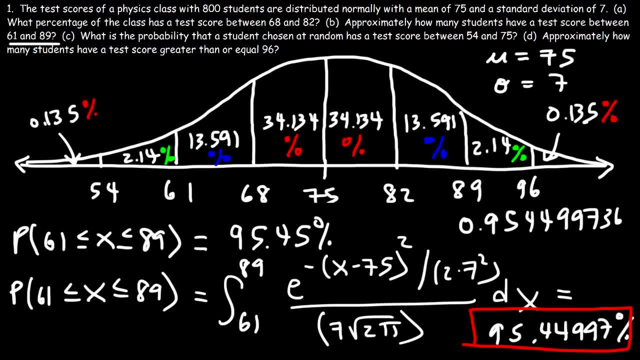 It rounds pretty well. Now, this is not the final answer for part b. So what's the answer for part b? So what this means is that 95.45% of the class has a test score between 61 and 89.. 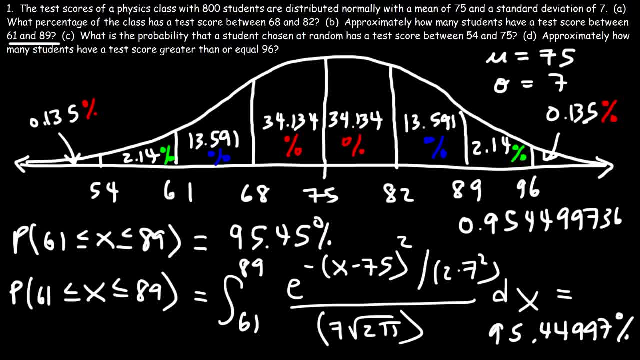 Now there's 800 students. So what's 95.45% of 800?? So what I'm going to do is take this number, because it's a more accurate value, and multiply that by 800.. My calculator also has a 1 here. 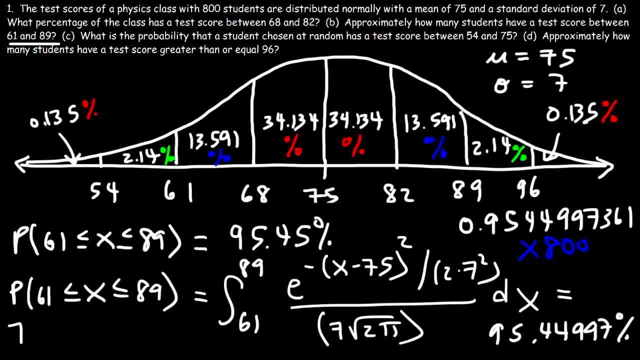 So if you take that number and multiply it by 800, it's going to give you 763.6, approximately. Now, because we're dealing with people, we want to round to the nearest whole number. So we're going to say approximately 764 students have a test score between 61 and 89.. 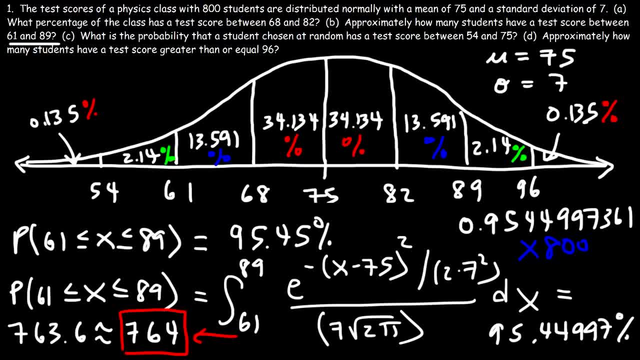 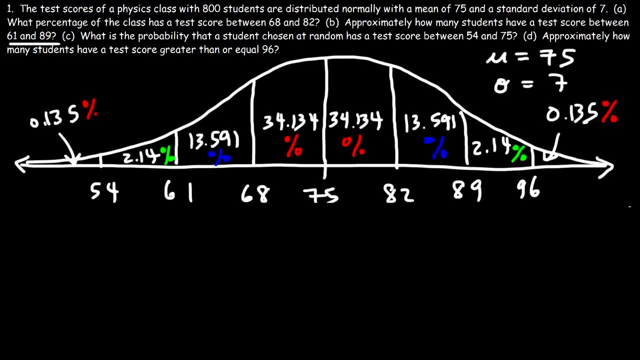 So this is the answer to part b. Now let's move on to part c. What is the probability that a student chosen at random has a test score between 54. and 75?? So go ahead and work on that problem. So here's 54, and we're going to stop at 75. 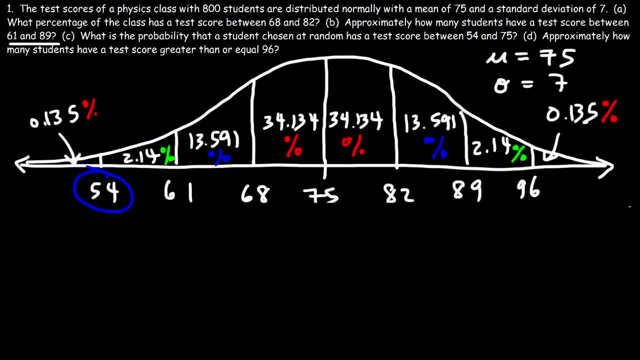 So basically we need to add these three numbers. So the probability of selecting a student that has a test score between 54 and 75 is going to be, So we're going to add 2.14 plus 13.5.. 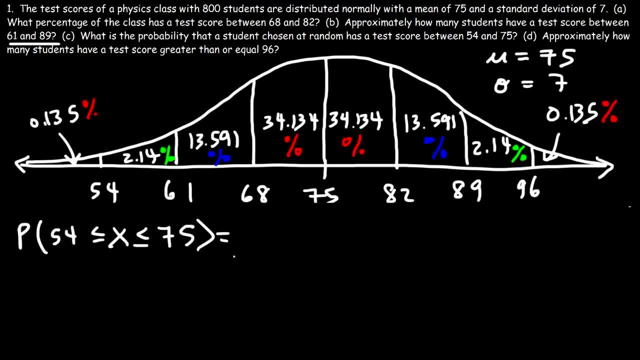 So 5.91 plus 34.134.. And so you should get 49.865%. So that's an approximation, pretty much a good approximation. Now let's get the exact answer, or a more accurate answer, using calculus. 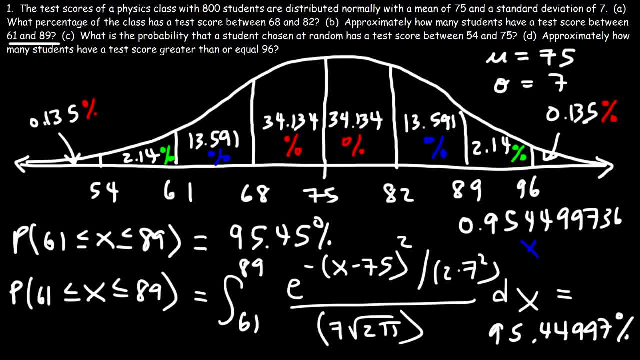 Because it's a more accurate value, And multiply that by 800. My calculator also has a 1 here. So if you take that number and multiply it by 800. It's going to give you 763.6 approximately. Now, because we're dealing with people, 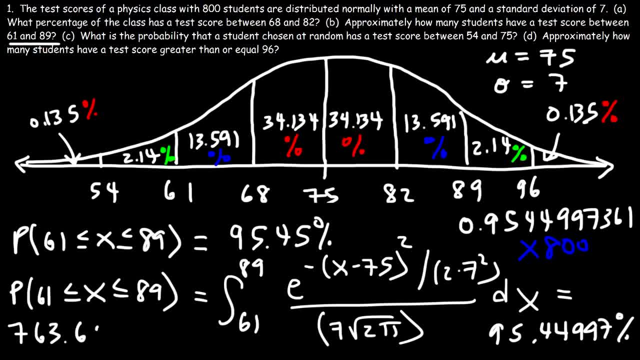 We want to round to the nearest whole number. So we're going to say approximately 764 students Have a test score between 61 and 89.. So this is the answer to part B. Now let's move on to part C. 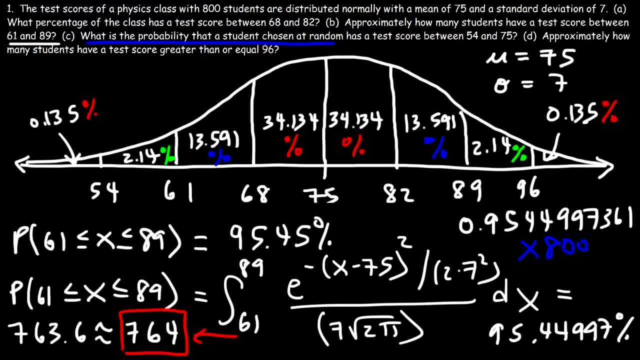 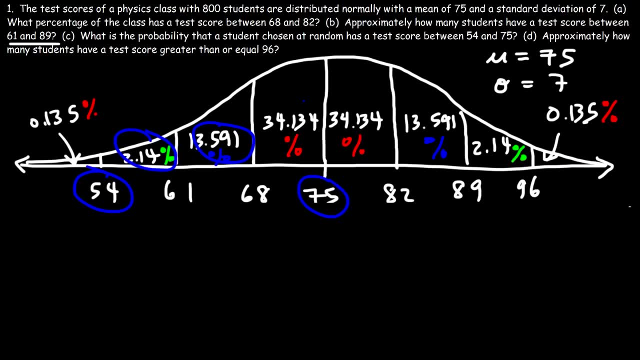 What is the probability that a student chosen at random Has a test score between 54 and 75?? So go ahead and work on that problem. Here's 54. We're going to stop at 75.. Basically, we need to add these three numbers. 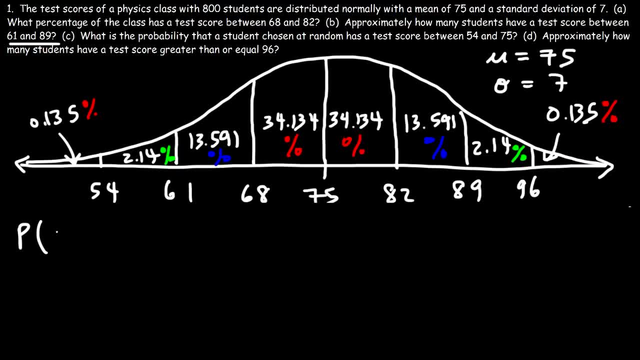 The probability of selecting a student that has a test score Between 54 and 75 is going to be, So we're going to add 2.14. Plus 13.591. plus 34.134, and so you should get 49.865 percent. so that's an approximation pretty. 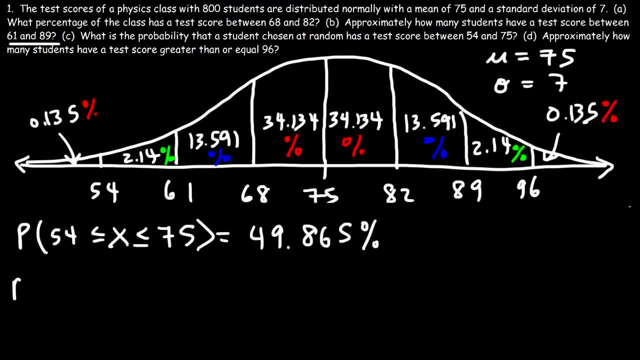 much a good approximation. now let's get the exact answer, or a more accurate answer, using calculus. so this is going to be the definite integral from 54 to 75: e negative x minus 75. let's not forget to square that divided by 2 times 7 squared. 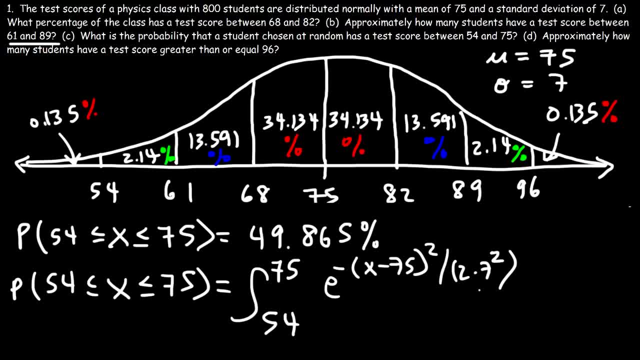 that's terrible looking too. i gotta fix that. divided by 7 times the square root of 2 pi dx and that's going to be 0.498650102, which is about 49.865 percent. if you want to get the exact answer, that's going to be 0.498650102. 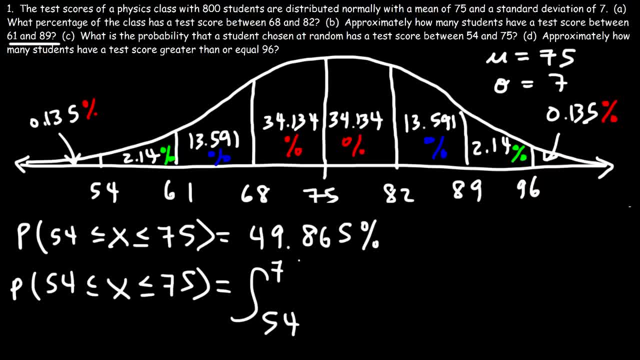 So this is going to be the definite integral from 54 to 75.. e negative x minus 75.. let's not forget to square that divided by 2 times 7. squared, that's terrible looking to fix that. divided by 7 times the square root of 2, pi DX. 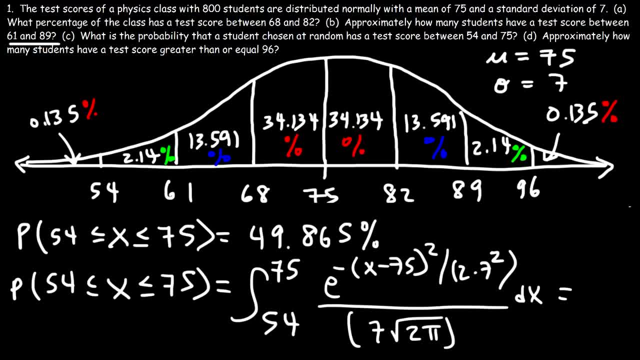 and so I got point four, nine eight, six, five, zero, one, zero two, which is about forty nine point eight, six, five, four percent. if you take this number and multiply by 100, so this is a very good approximation, and so that's the answer for Part C. 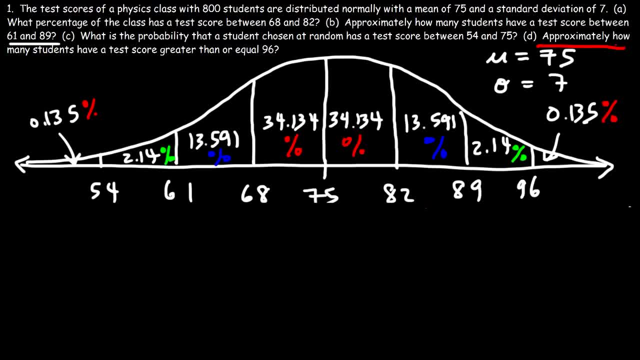 Part D, the last part of the problem, approximately how many students have a test score greater than or equal to 96? so, using a graph, what's the answer? so all we need is this region, which we can clearly see, that it's point one, three, five percent. now we're not looking for. 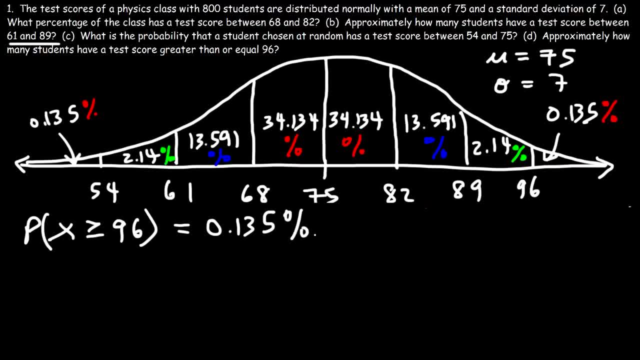 the percentage, but the number of students, which we'll get to later. so how can we get the same answer using calculus? so we know we need to calculate the definite integral from A to B. now we can see that a is 96, but we only have one number here. so what to be? what should we put for B? now if 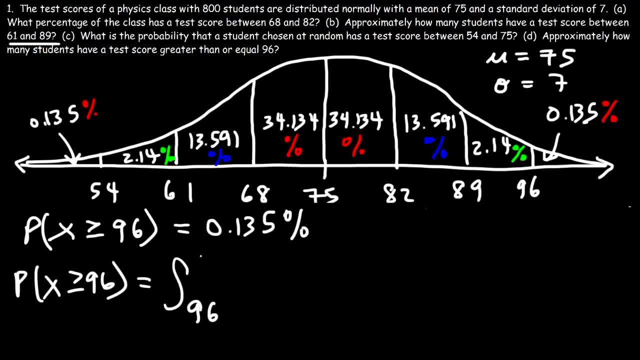 you're thinking of a hundred. you shouldn't use that because, Granson, most head scores are graded based on a hundred percent, like. the highest value is one hundred, but sometimes teachers may have extra credit, so some students could have a a score of 105 or 110. if you put a hundred here, you won't get a. 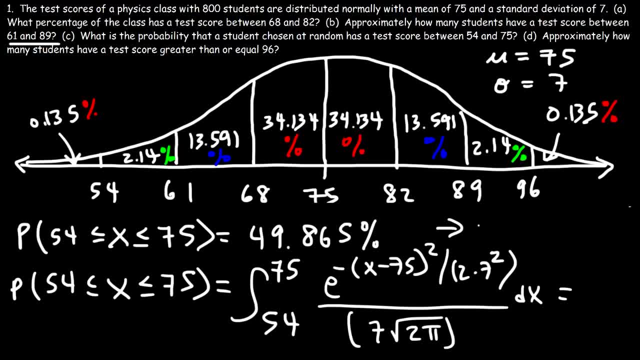 and so i got 0.498650102, which is about 49.865 percent. if you want to get the exact answer, that's going to be 0.498650102. take this number and multiply by 100, so this is a very good approximation. 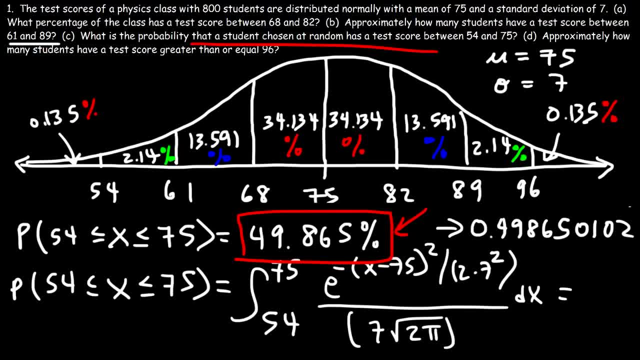 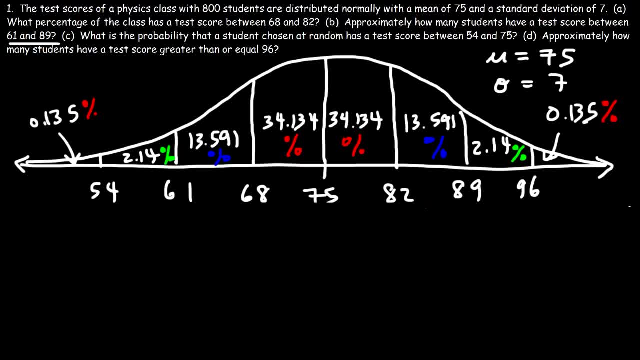 and so that's the answer for part c. part d, the last part of the problem, approximately how many students have a test score greater than or equal to 96.. so, using the graph, what's the answer? so all we need is this region, which we can clearly see that it's 0.135. 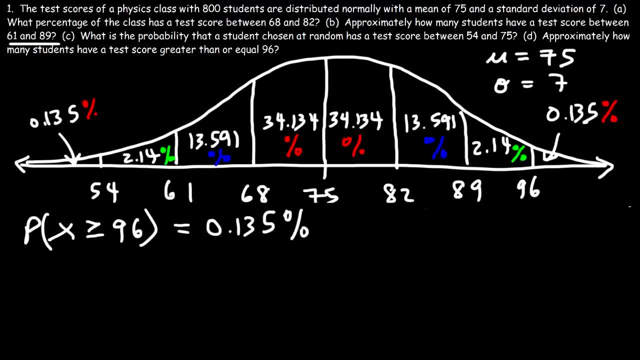 now we're not looking for the percentage but the number of students, which we'll get to later. so how can we get the same answer using calculus? so we know we need to calculate the definite integral from a to b. now we can see that a is 96. 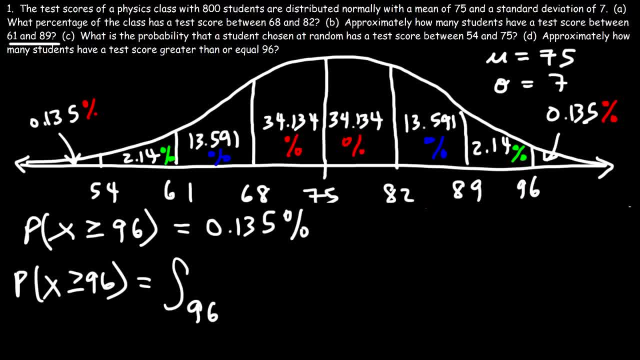 but we only have 1.95 number here. so what's B? what should we put for B? now, if you're thinking of a hundred, you shouldn't use that because, granted, most test scores are graded based on a hundred percent, like the highest value is 100, but sometimes 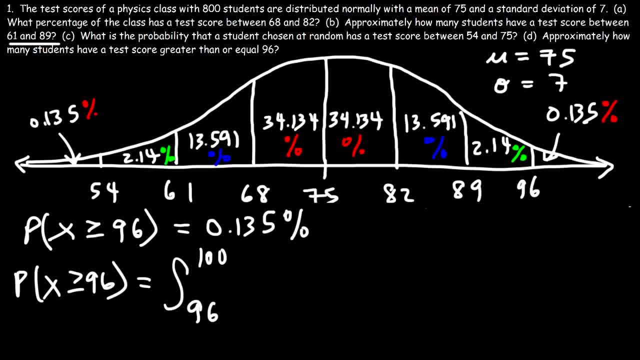 teachers may have extra credit, so some students could have a score of 105 or 110. if you put a hundred here, you won't get point one, three, five percent. let's call the function f of X. instead of writing the whole thing, I'm gonna plug. 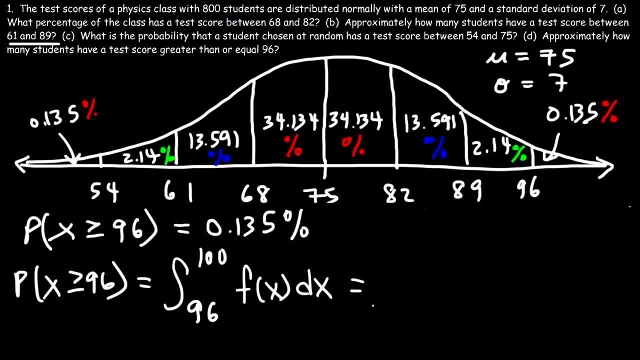 it in. so give me one minute to do that. and so if you integrate it from 96 to 100, you're going to get point zero, zero, one, one, seven, two, three, eight. so if you multiply that by a hundred, that correlates to point one one seven percent approximately, which is not the 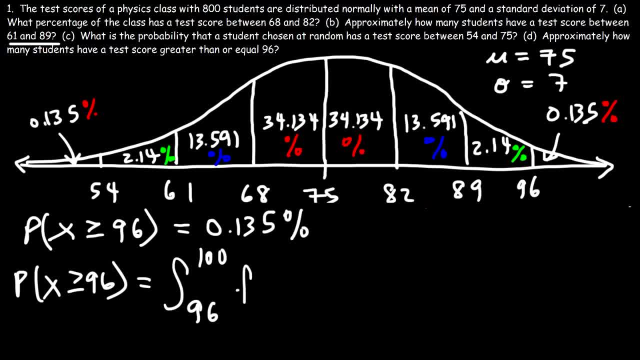 at 0.135%. Let's call the function f of x. instead of writing the whole thing, I'm going to plug it in. Give me one minute to do that. If you integrate it from 96 to 100, you're going. 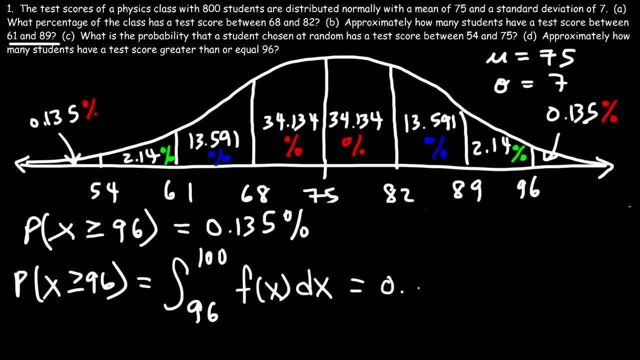 to get 0.001%. So if you multiply that by 100, that correlates to 0.117% approximately, which is not the same as this answer. So what you need to keep in mind is that this goes to infinity, and 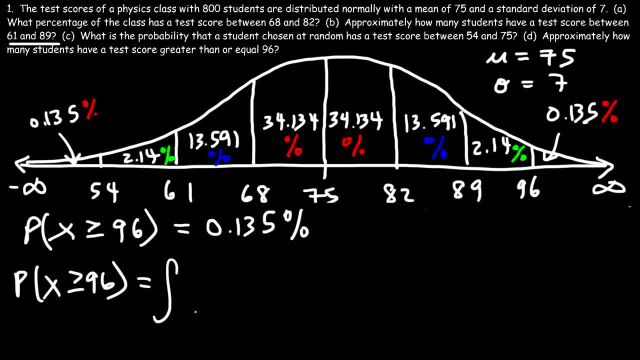 the left side goes to negative infinity, So you have to integrate it from 96 to infinity. Okay, Now this is going to be a problem because for the most part, we can't plug in infinity into a calculator. So we can approximate the answer by picking a number. that's I need. 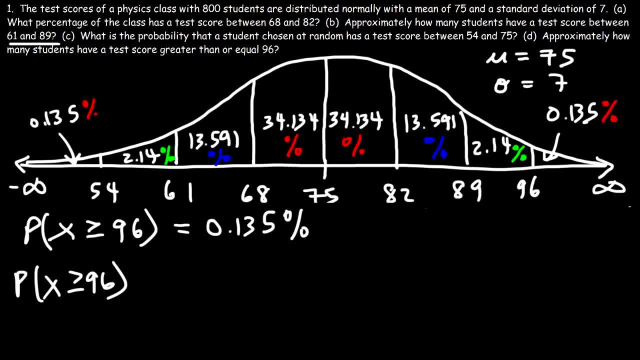 to get rid of this, We need to pick a number that is very high, that can represent infinity. So 100 wasn't good enough, so let's pick a much bigger number, like 1,000.. So we're going to do that. 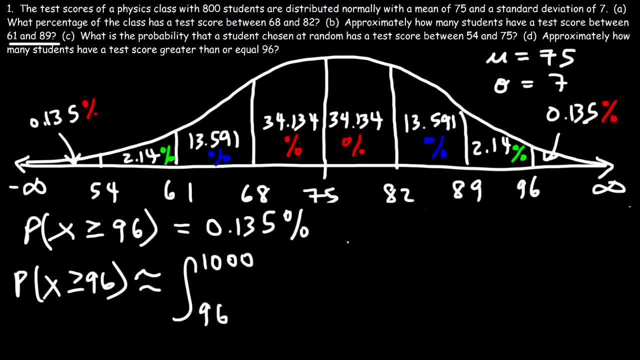 Now the answer won't be exact, but it's going to be a very, very good approximation. So if you go ahead and plug this in, you should get an answer that's very, very close to this answer. So go ahead and type that into your calculator. Now my calculator gave me this answer: 0.001%. 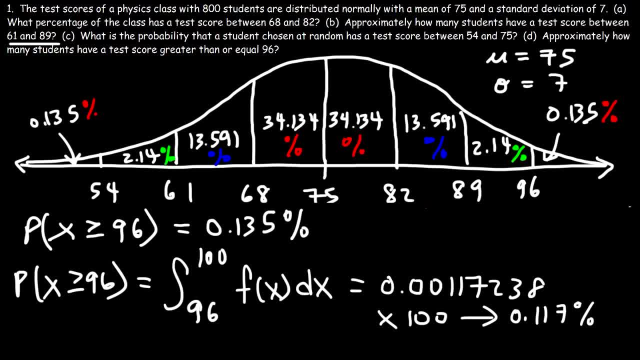 same as this answer. so what you need to keep in mind is that this goes to infinity and the left side goes to negative infinity, so you have to integrate it from 96 to infinity. now this is going to be a problem because, for the most part, we can't plug in infinity into a calculator. 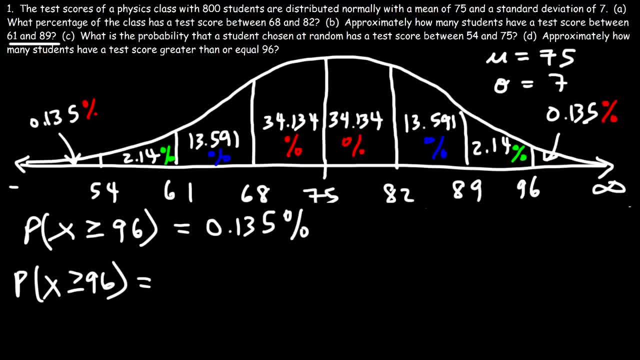 so we can approximate the answer by picking a number, that's. I need to put a number on the right side to get rid of this. we need to pick a number that is very high, that can represent affinity. so a hundred wasn't good enough, so let's pick a much bigger. 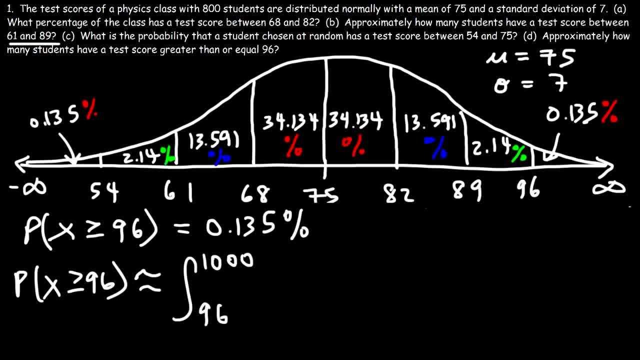 number like a thousand. now the answer will be exact, but it's going to be a very, very good approximation. so if you go ahead and plug this in, you should get an answer that's a very, very close to this answer. so go ahead and type that into your calculator now. my calculator gave me. 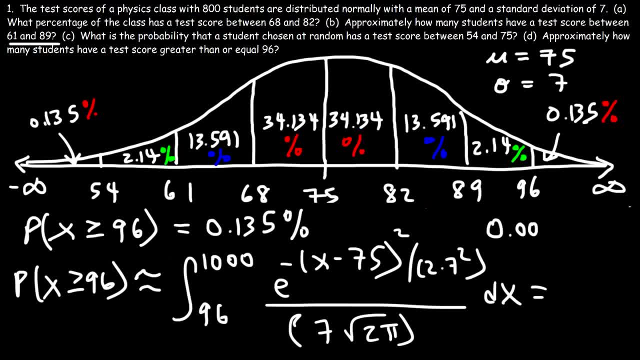 this answer: point zero, zero, one, three, four, nine, eight, nine, zero three. so multiply that by a hundred and that's about point one, three, four, nine, eight, nine and I'll stop there- percent. so this rounds to point one, three, five percent. so that's a good approximation. 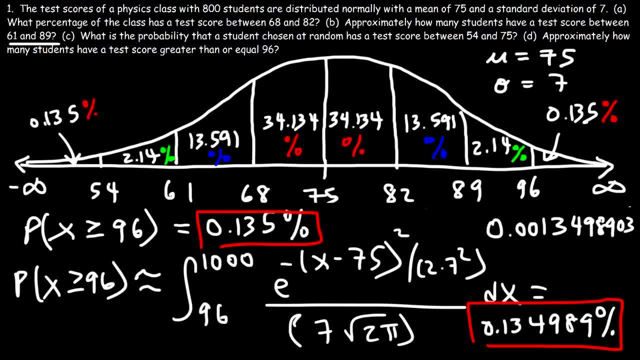 now let's determine the number of students that have a test score that's equal to or greater than ninety six. so we're going to take this number and multiplied by the number of students in class: 802 point zero, zero, one, three, four, nine, eight, nine, zero, three times 800 you. 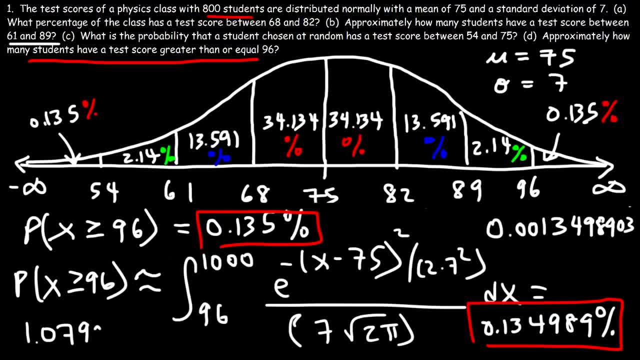 should get 1.0799, and so for this we're going to round it to the nearest whole number. so approximately one student scored a 96 or more on his physics exam. So that's how you can use the normal distribution curve to answer problems. 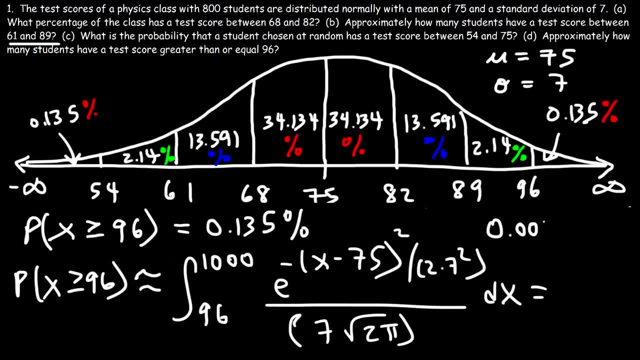 Okay, So I'm going to plug this in. Okay, So this is going to be 0.0013498903.. So multiply that by 100, and that's about 0.134989, and I'll stop there. percent. 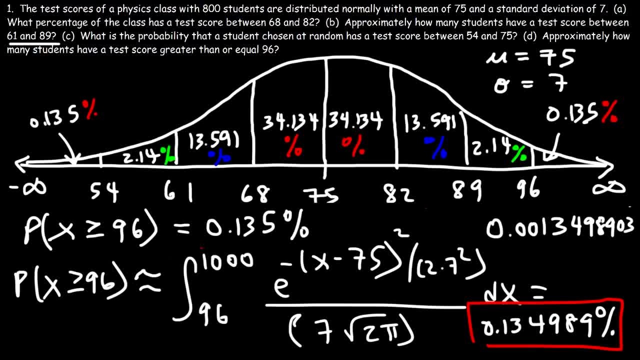 So this rounds to 0.135%. so that's a good approximation. Now let's determine the number of students that have a test score that's equal to or greater than 96.. So we're going to take this number and multiply it by the number of students in class: 800. 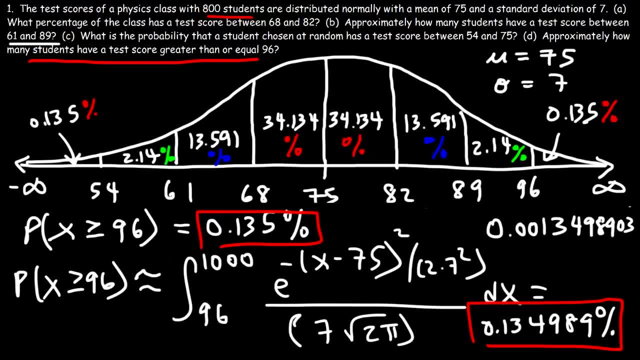 So 0.0013498903 times 800, you should get 1.0799.. And so for this we're going to round it to the nearest whole number. so approximately one student scored a 96 or more on his physics test. 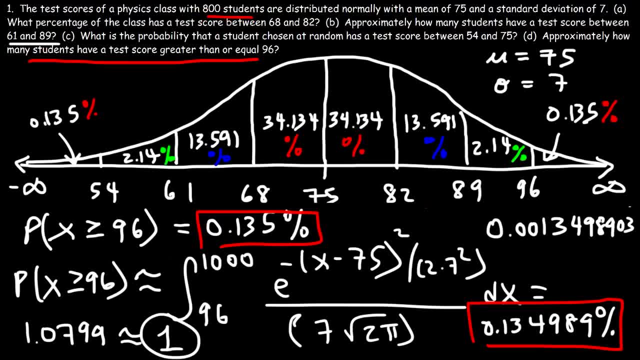 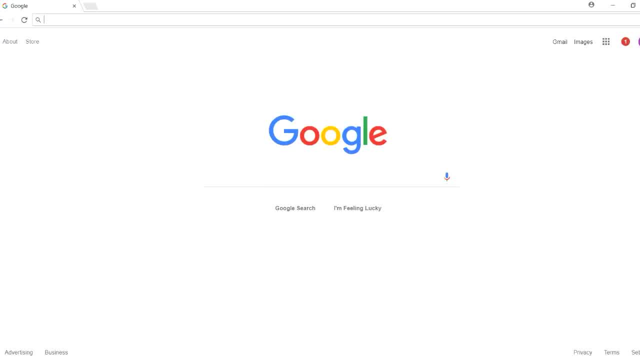 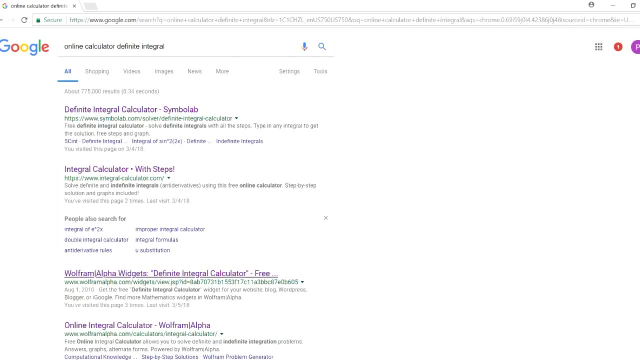 So that's how you can use the normal distribution curve to answer problems such as this one. Now go ahead and open up your internet browser- I'm going to use the Google search engine- and then, when you're ready, type in online calculator: definite integral. and then you can also type in Wolfram Alpha. 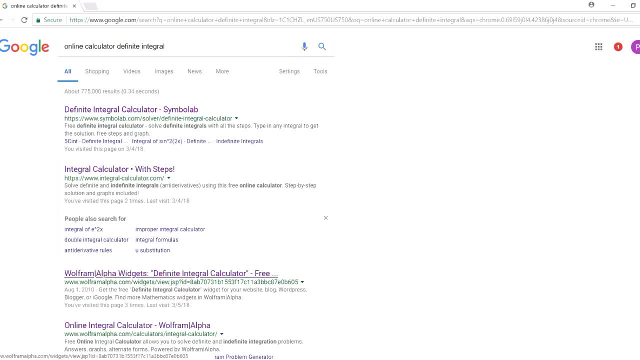 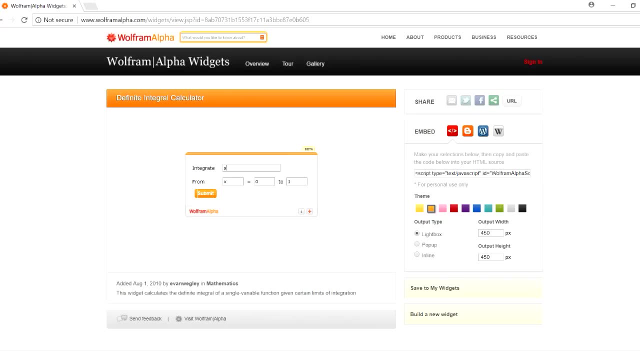 So I'm going to go to this site: Wolfram Alpha Widgets definite integral calculator- Okay, And you should see a page that looks like this. So type it in exactly the way I'm going to show it to you. So type in E and then shift 6 to get the arrow, negative parentheses. 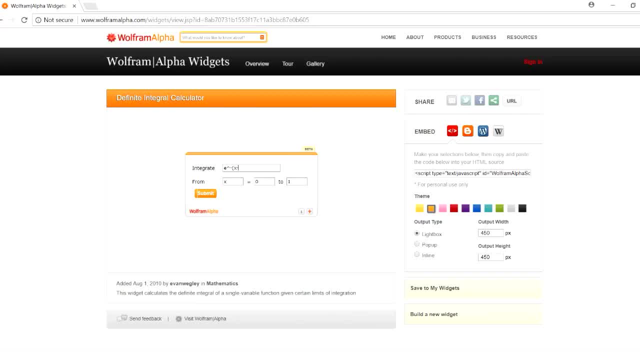 If you don't put the negative sign, you will get it wrong. X minus 75 squared, that's shift 6, and then we also need to open up another parentheses in front of the negative sign. So you need to open it up. 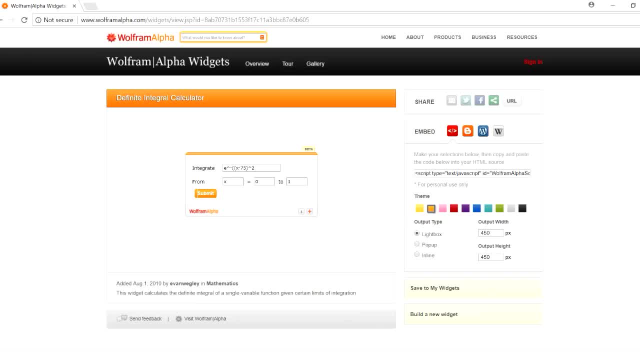 So you need to open up two parentheses. keep that in mind And then divide it by open a new parentheses. 2, shift 8, that's the multiplication symbol times 7, squared, Close parentheses and close it again. This entire thing has to be on the exponent of E. That's why we have to open up an additional. 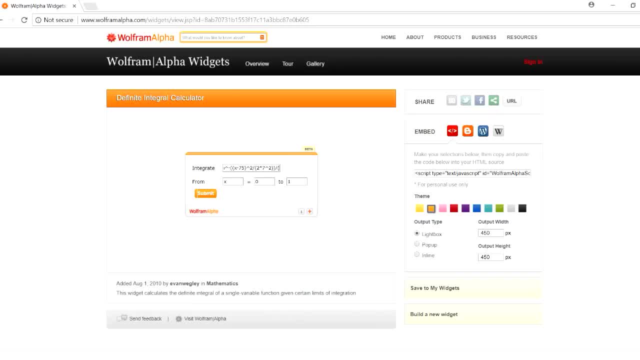 set of parentheses And then divide it by open a new set of parentheses, 7 square root SQRT, That's 7 squared. Open parentheses again, 2 pi, 2 pi and then close the parentheses twice. Now we're going to integrate it from 68 to 82.. 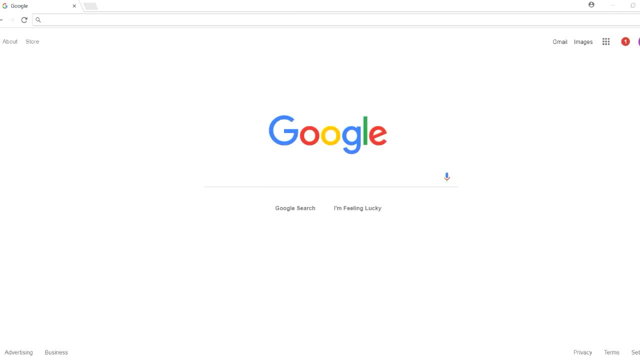 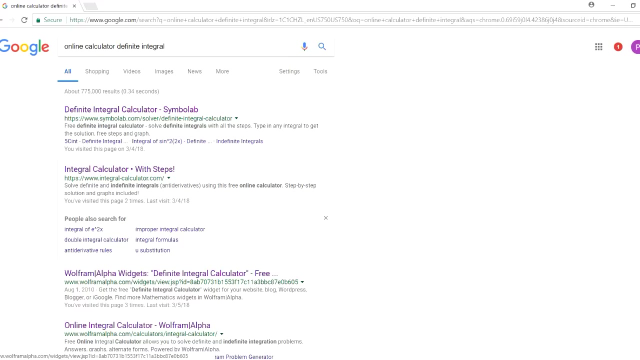 such as this one. Now go ahead and open up your internet browser. I'm going to use the Google search engine and then, when you're ready, type in online calculator: definite integral. and then you can also type in Wolfram Alpha. So I'm going to go to this site: Wolfram Alpha widgets- definite integral. 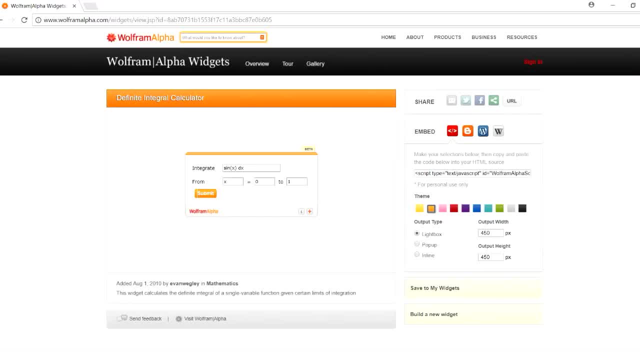 calculator and you should see a page that looks like this. So type it in exactly the way I'm going to show it to you. So type in E and then shift 6 to get the arrow negative, negative parentheses. if you don't put the negative sign, you will get it wrong x. 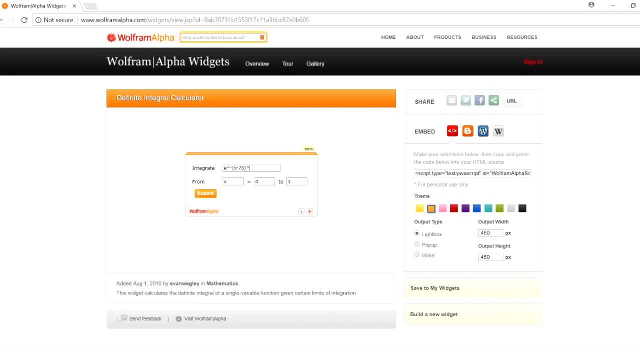 minus 75 squared, that's shift 6. and then we also need to open up another parentheses in front of the negative sign. So you need to open up two parentheses. keep that in mind and then, divided by, open a new parentheses 2, shift 8. that's the. 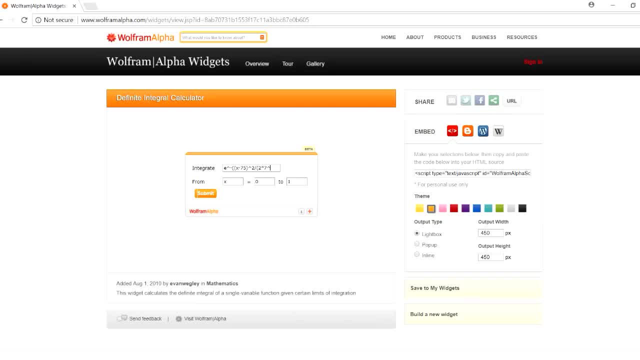 multiplication symbol times 7 squared. close parentheses and close it again. This entire thing has to be on the exponent of E. That's why we have to open up an additional set of parentheses and then, divided by, open a new set of parentheses: 7 square root, sqrt. open parentheses again: 2 pi, 2 pi, and then. 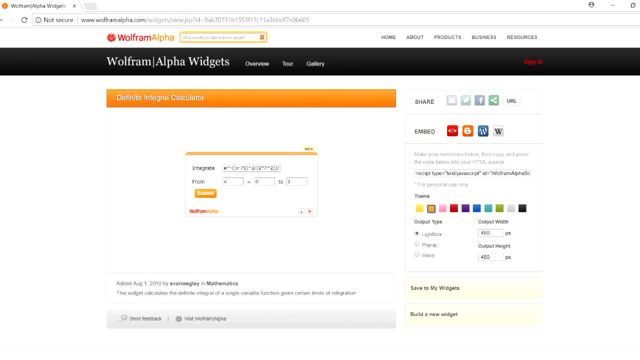 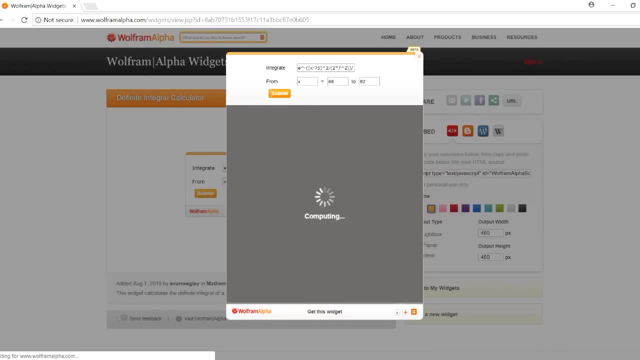 close the parentheses twice. Now we're going to integrate it from 68 to 82 and then click Submit So you can see the answer here: 0.682689, so that's about 68.269 percent if you multiply it by 100.. Now the good thing about this is you don't need to type in. 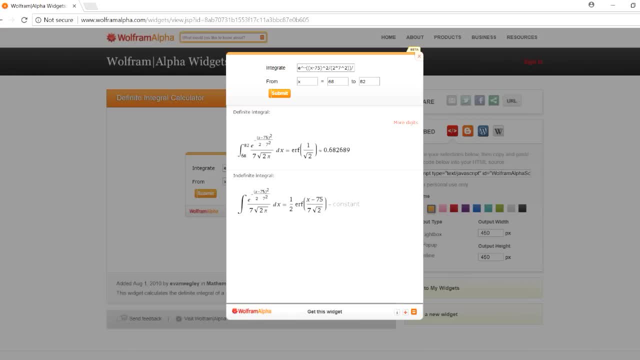 the integral expression, because that part is not going to change. The only thing you need to change are the limits of integration. So for part B we need to find a probability from 61 to 89. So let's change these numbers and then. 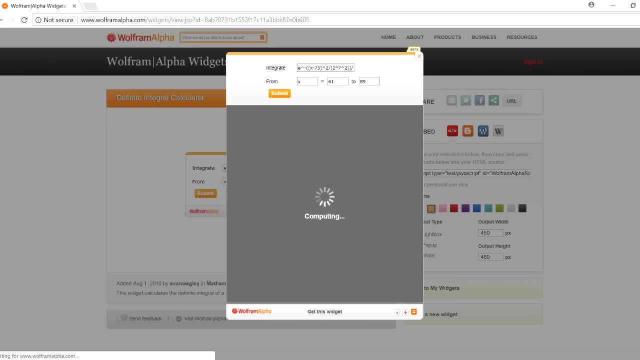 just click Submit, And so we have 0.9545.. If you need more digits, click the more digits link here and then you can get a more accurate answer, which we had: 0.9545.. and then you can get a more accurate answer, which we had 0.9545.. 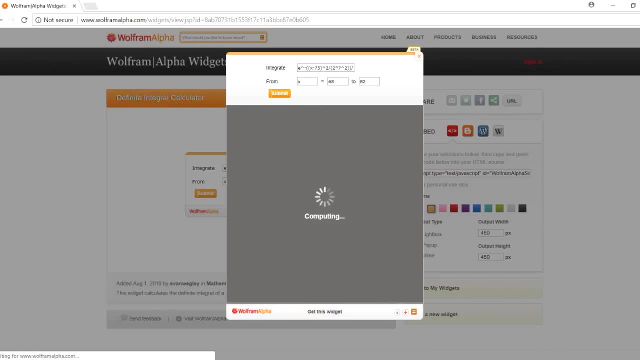 And then click submit So you can see the answer here: 0.682689.. So that's about 68.269 percent If you multiply it by 100.. Now the good thing about this is you don't need to type in the integral expression. 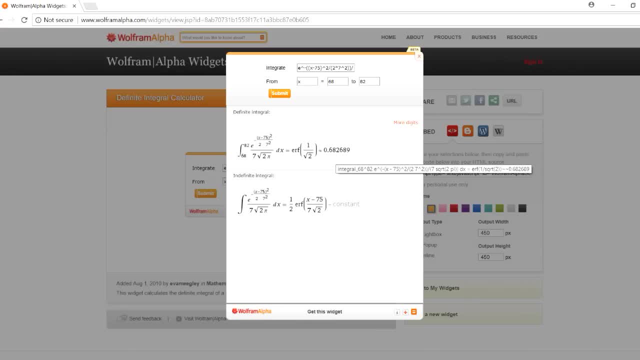 Because that part is not going to change. The only thing you need to change are the limits of integration. So for part B we need to find a probability from 61 to 89. So let's change these numbers And then just click submit. 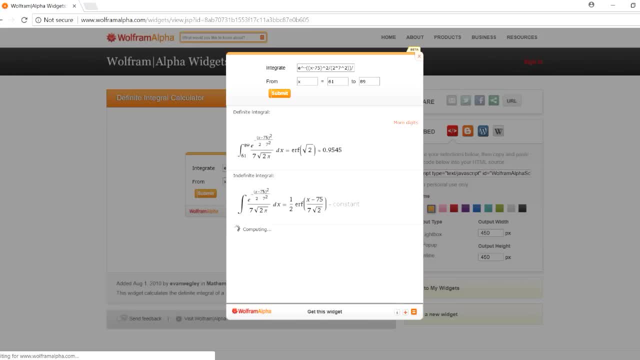 And so we have 0.962689.. Okay, We have 0.9545, or 95.45 percent. If you need more digits, click the more digits link here And then you can get a more accurate answer, Which we had: 0.9544997.. 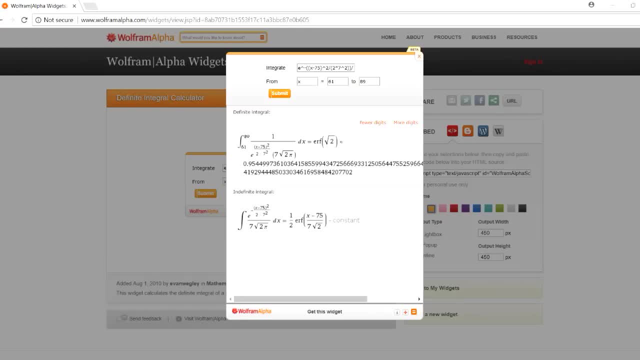 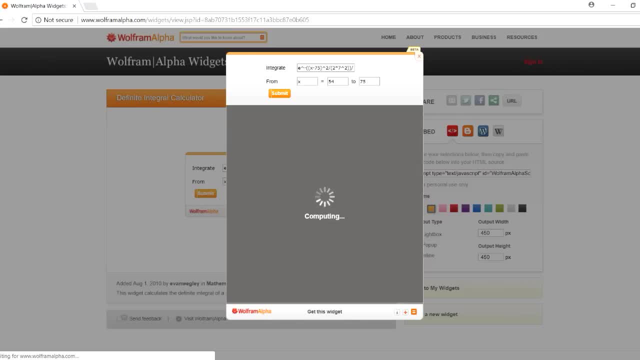 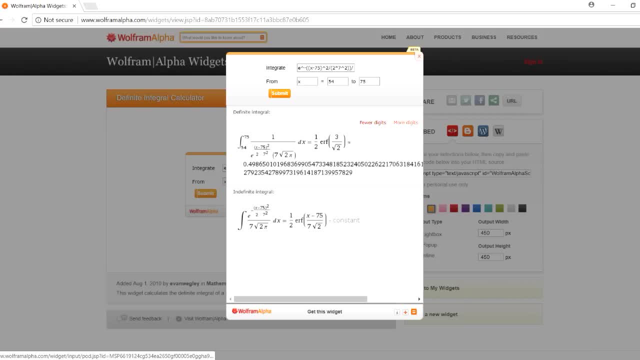 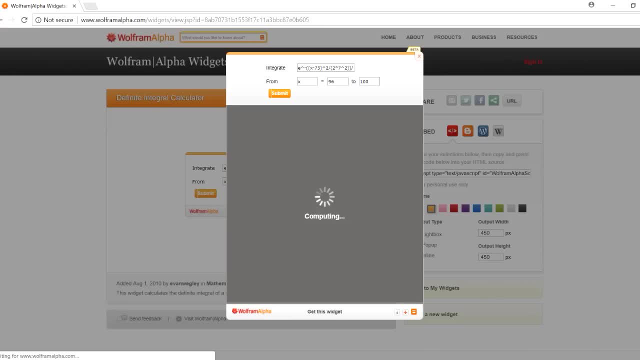 one, three, five percent. you need to go to infinity. so, as you can see, point zero zero one, one, seven. so this is not an accurate answer. but as you increase this value, let's say to 105, it's going to approach a more accurate answer. notice point zero zero one, three, four. so it's getting close to point zero zero one. which we had 0.9545.. which we had 0.9545.. and then you can see that there's 2.945%. So you need 5.425, 0 and an 8.���reiw играj identifier and then you print out. And so you can see that there's three other, beispielsweise those numbers like program 2, I'm going to print them out, and surprised Is Obviously. examples show the two tres that provide 0.9545 for five plus 4.. The other ones are important here. 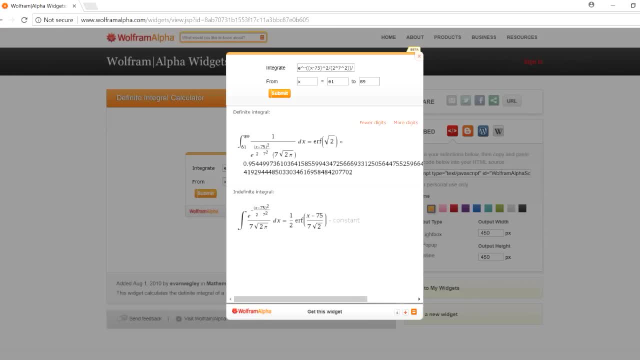 And so these other ones have some changes here, And if you want more numbers beyond that, you can write to your heart's pleasure. Now let's move on to Part C. So it was from 54 to 75. And so we did get this answer- 0.49865,, and to see a more accurate answer, 0.4986501,. 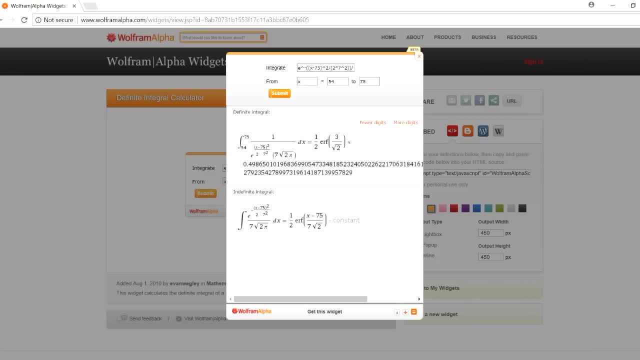 and we rounded it to 02, at least my calculator did that. But we can leave it as 0.49865, or 49.865%. Now for the last one. now, I mentioned not to integrate it from 96 to 100, because it 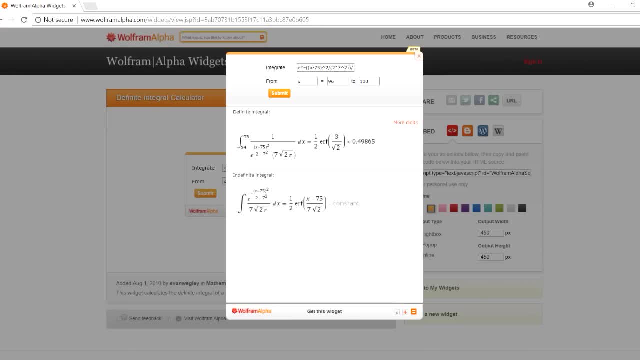 won't give you 0.49865.. You need to go to infinity, So, as you can see, 0.00117.. So this is not an accurate answer, But as you increase this value, let's say, to 105, it's going to approach a more accurate 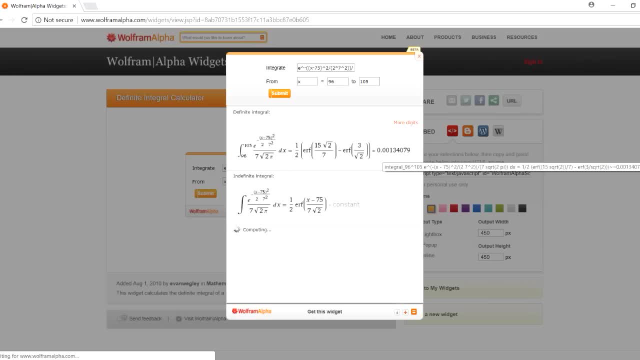 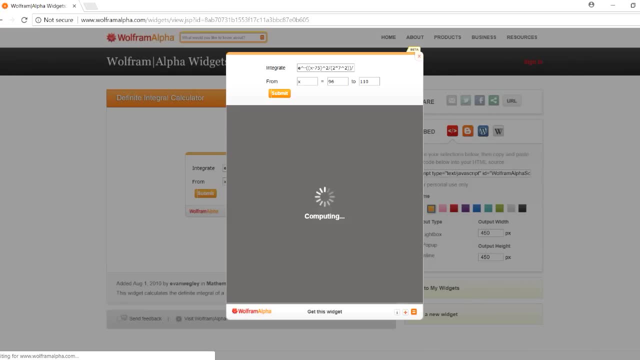 answer: Notice 0.00134.. So it's getting close to 0.00135.. So let's try 110.. Now, if you want to increase this value, you need to go to infinity. Notice 0.00134.. 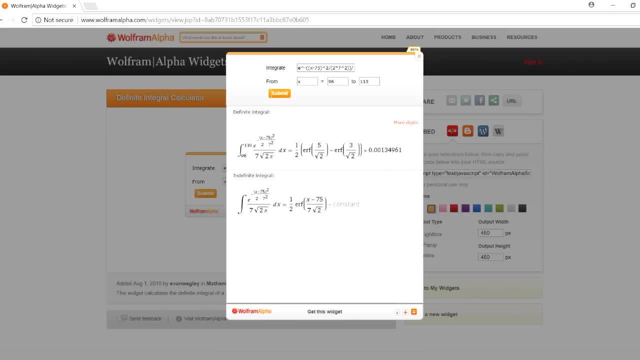 Now notice that it's converging. it's getting closer to 0.00135.. So we'll need to pick a large number that represents infinity. So we can try 1,000.. So we get 0.0013499.. 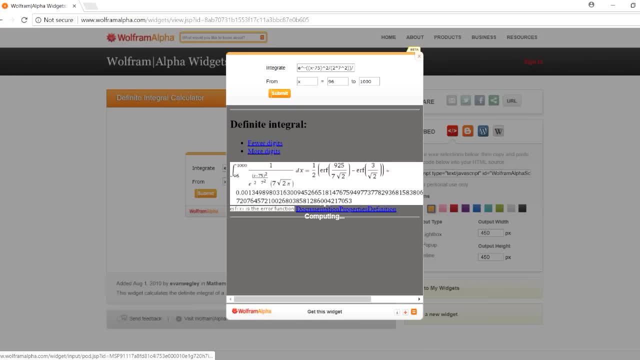 And you can select more digits if you want. Now let's pick a number that's bigger than 1,000. To see if it's going to stay at this value, if it's going to converge to it. If the value changes, then we don't have the right answer.